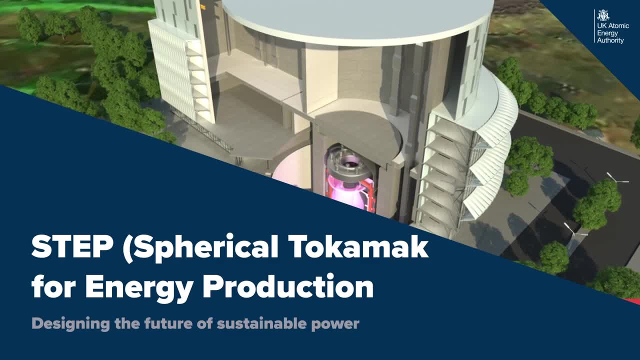 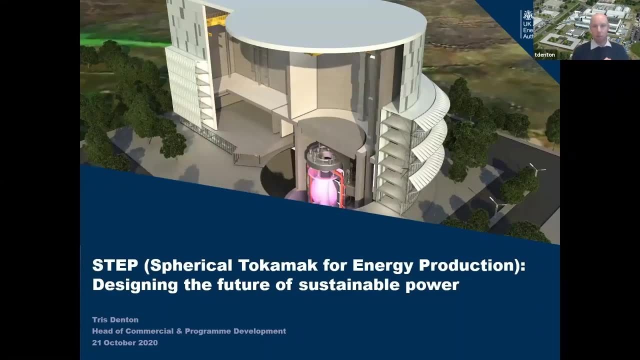 Okay, look folks, good afternoon. My computer's telling me it's 1.30.. My watch is telling me it's 1.31, so I think it's good time to get going on the webinar today. Listen first. 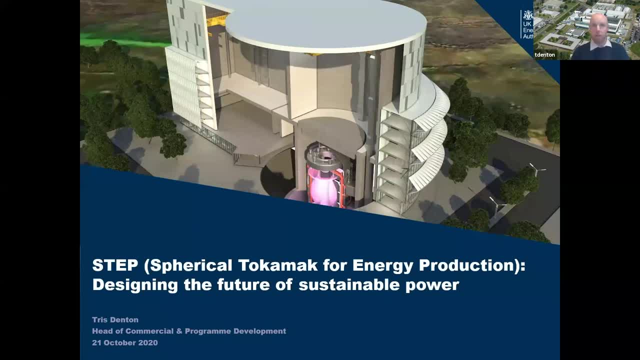 and foremost, thank you very much. People giving up an hour of their day to hear from the programme is always a bit humbling. We really hope we can make a good use of your hour, especially when that hour's at lunchtime. So I promise I'll try and do the decent thing. 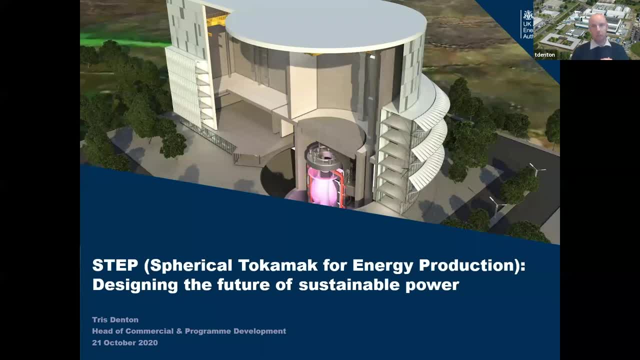 and keep it all very, very interesting. The style I'm going to take today is going to be pretty casual. I think that facilitates the most interesting conversation You know. I'd like this to feel much more like we're all sat around a table having a giant lunch. 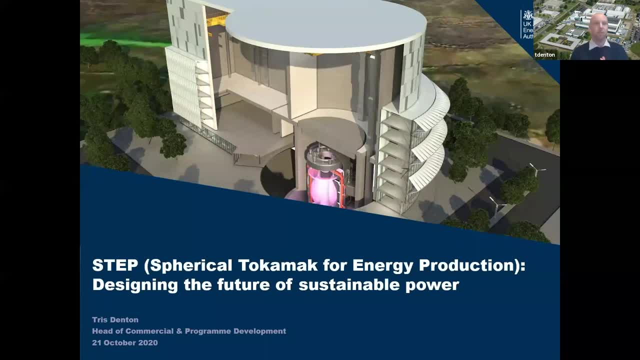 together rather than sat in sort of stuffy formal proceedings. You know, I think we'll have just the most enjoyable time that way. What I'm going to do, I'm going to talk for about 20 minutes or so- hopefully less, and 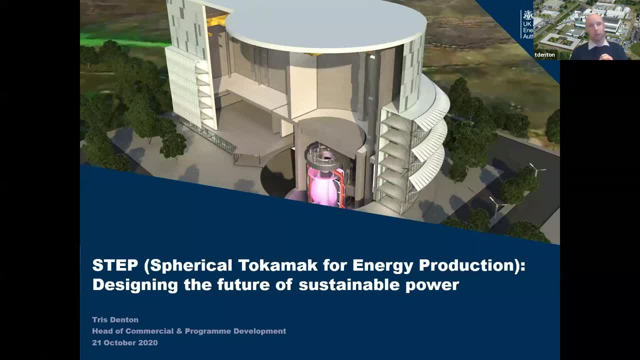 leave the rest of the time open for Q&A. I presume most folks are familiar with the platform by now, working with Zoom, but just type questions into the Q&A box. I'll come on to those at the end, If we do run out of time, which I hope we won't, but if we do run out of time. 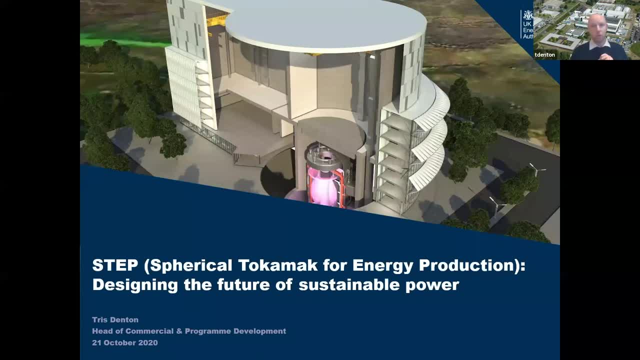 at the end of this presentation I'll share some contact details where you can send on further questions to colleagues in our corporate comms team, And we can also use that if there are any that I can't answer on the hoof today, I promise. 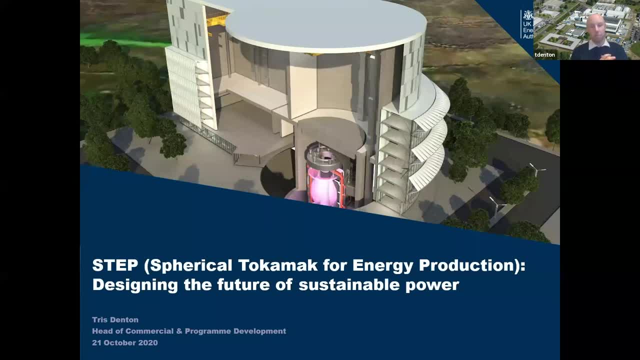 you. I'll do my very level best, But there's always- you know always- ones where I need to draw on the fantastic body of resource we've got within the authority. The other thing I'd like to offer today is to UKAA's corporate comms team Facilitating events. 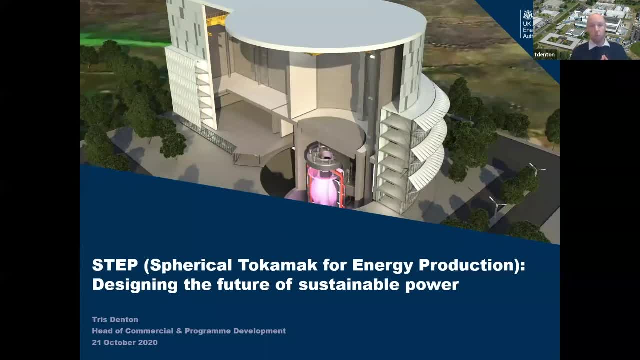 like this. getting everything ready, getting everything set up, really is a huge amount of work on their part. They really do throw themselves into it, And I'd like to thank them for giving me the chance to speak with all of you. So before I do anything else, I'll introduce myself. My name is Tris Denton. I'm the head. 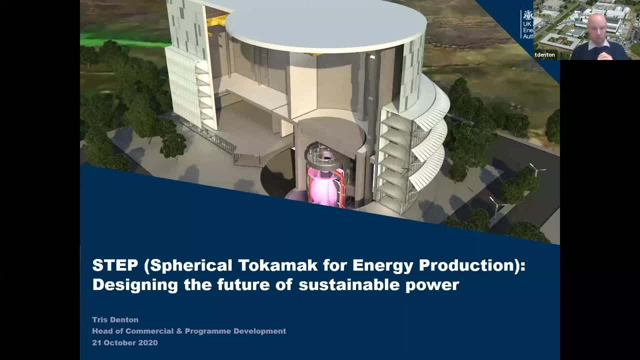 of commercial and program development for STEP. I'm trying to break that job title down so you can understand where I'm coming from, what I'm doing. I'd like to summarize: I'm doing everything except designing a tokamak. Sometimes I have to say my degree is in politics. 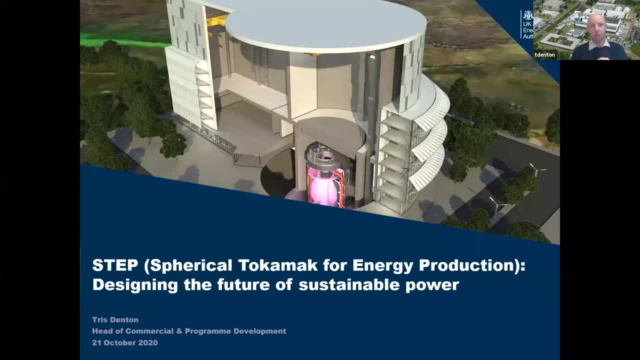 and I've already seen on the chat there's folks here with far more technical engineering fusion qualifications than I am, So I'm not going to try and teach you all about the detail of the inner workings of spherical tokamak, What I hope I can do and what I 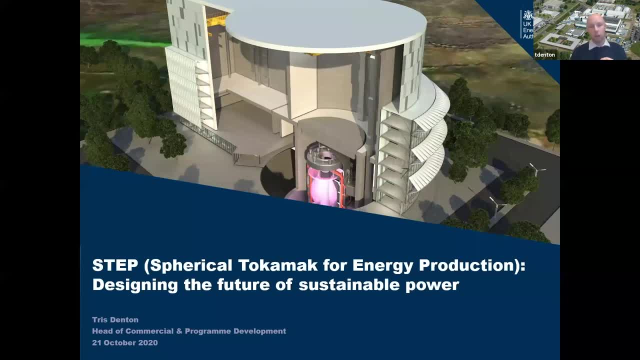 hope is interesting is to talk a bit about the program. we have to deliver across the full scope the program, working with stakeholders, working with industry, working with academia, working with government, working with regulators, seeking to bring forward a really credible program: not just design the equipment, but bring forward a full-scale, spherical tokamak. 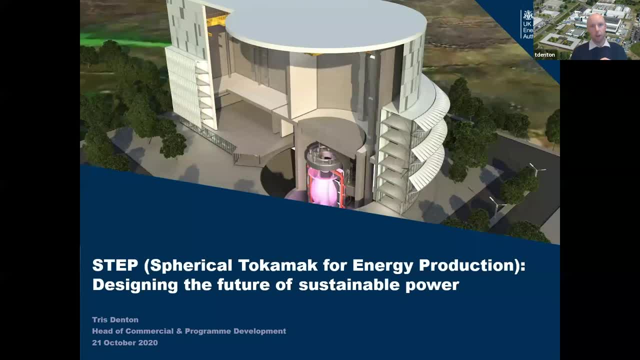 for energy production And I hope I can cover that in the next few days. So thank you very much. I'll see you in a few minutes. The other thing I want to do while I'm on the title slide, and I don't know if this: 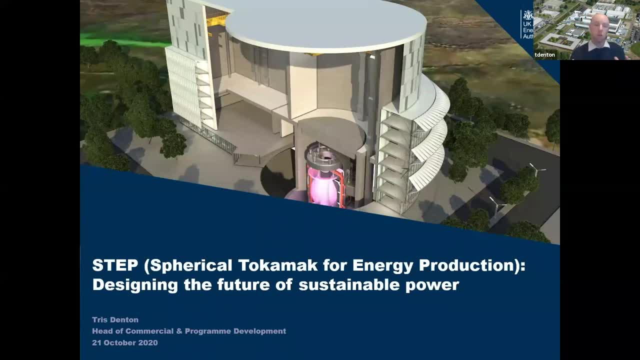 is normal at these webinars or not is when we're working in step in our meetings. we tend to start sessions with a safety or wellbeing or culture moment. Just take a moment to reflect on how we're all doing and what we all need. Obviously, in normal times, I'd be telling. 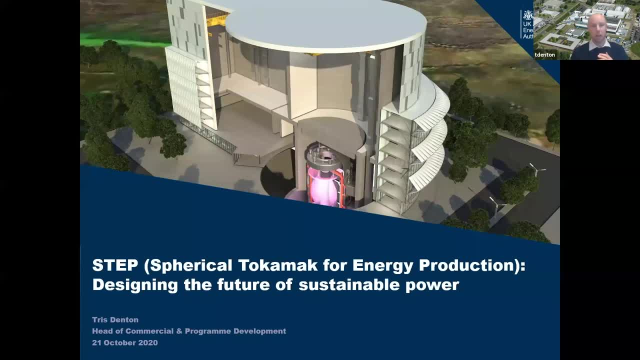 you please turn off your phones, and here's the fire exits. I can't do that. What I can say is that one of the things we've been looking at lately as we start meetings is just being aware that current working arrangements can be tough for all sorts of different reasons. 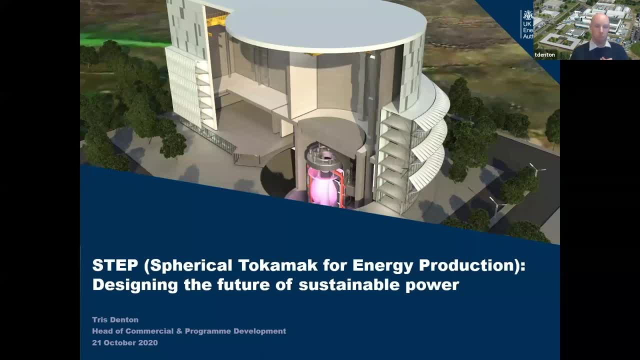 Some people are finding it lonely, Some people haven't got a great space to work, And what we're certainly trying to do is just look out for our teammates, look out for our mates, make sure we're all okay, Keep an eye on the people we're working with around us, So just 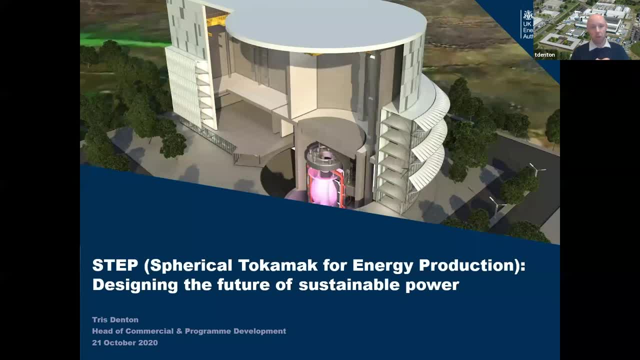 take a moment here. I hope everyone on this call is doing okay, And let's look after one another while we're working in slightly unusual ways. Okay, Okay, So this webinar is going to be recorded. You're wonderfully invisible. I can't see. 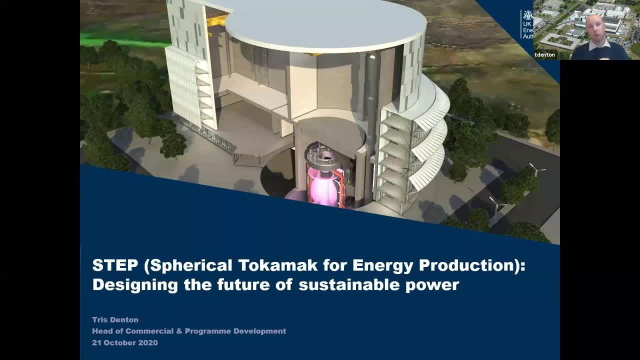 you. The recording can't see you. It can see me and it will be shared on our YouTube platform. The question and answer function doesn't show on that recording, So please do feel free still to ask me questions, as you usually would. Okay, 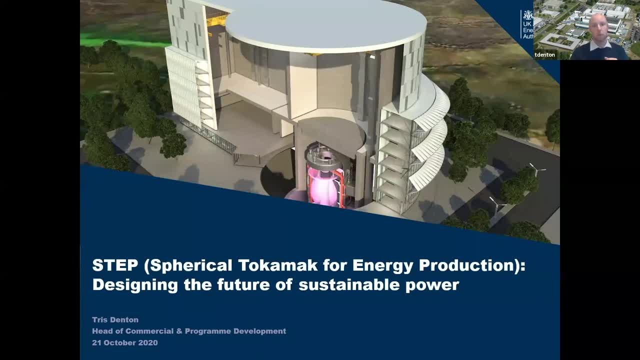 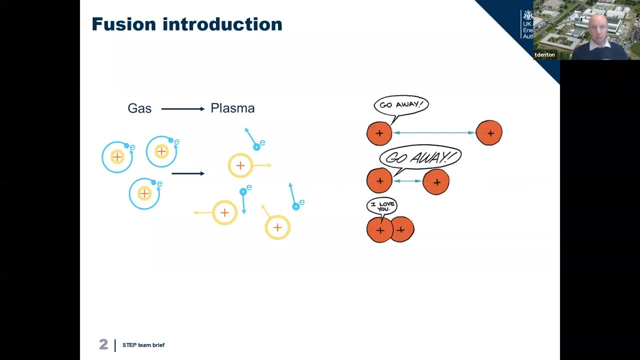 I can take the slides forward. So, Fusion, like I say, there's people on this call who don't understand the detail of this far better than I, but let me give you a non-technical perspective on the challenge we face as a Fusion industry and as a STEP program. We 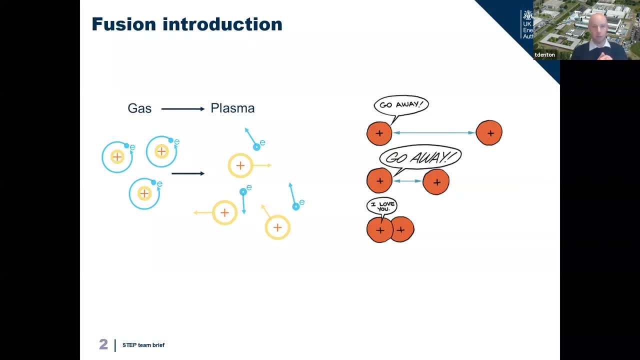 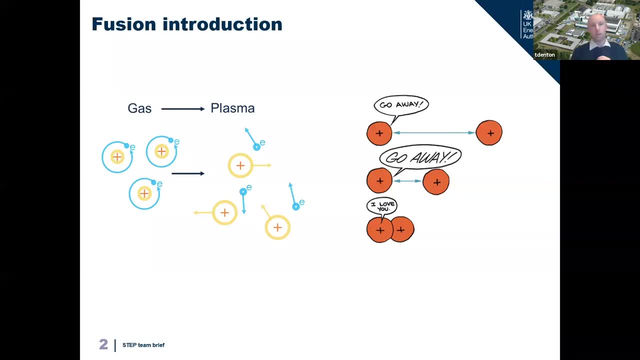 you that I've been working in Fusion for 18 months or so and I can tell you that when I first visited Cullum and looked at JET, it is awe-inspiring, It's fantastic, The story it tells is incredible And, as a sector, I think we should never lose that and I hope. 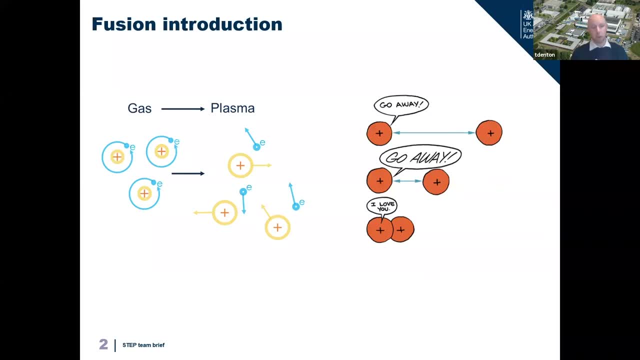 all the folks listening to this who aren't part of the sector will share that view and increasingly be captured by the excitement and the possibilities that this offers. The challenge, of course, is to harness Fusion as a useful, deployable, commercially viable source of energy for humanity. 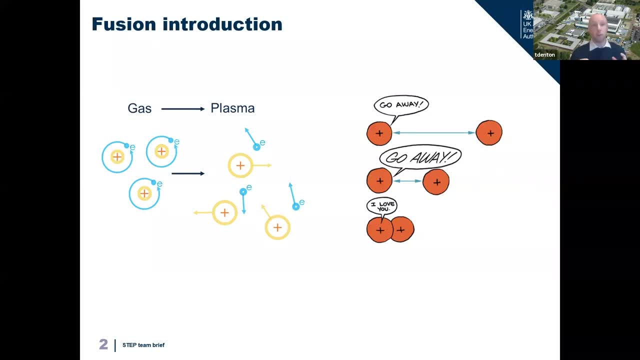 That's why when we talk about STEP, the Spherical Tokamak for Energy Production- we've named that advisedly. We really are focused that this plant must deliver net energy and be an effective demonstration prototype to pave the way for a successful fusion plant. 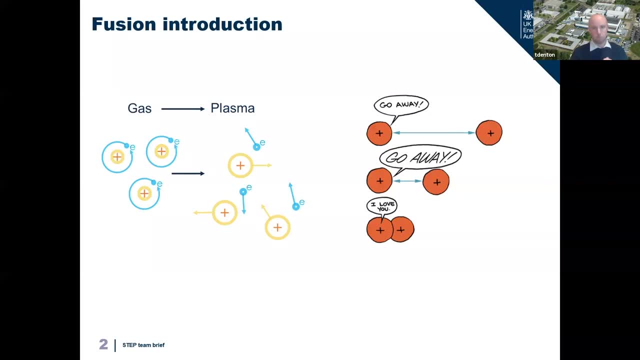 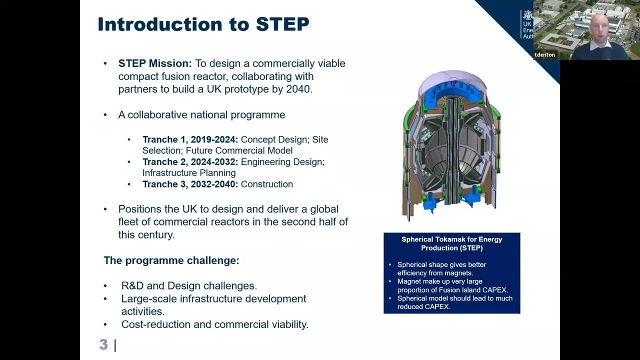 on the grid, here and elsewhere. Introduction to STEP. So, as I say, we're the Spherical Tokamak for Energy Production programme with a mission to design a commercially viable compact fusion reactor. It's a very clear mission, It's a very ambitious mission, It's a very exciting mission. This. 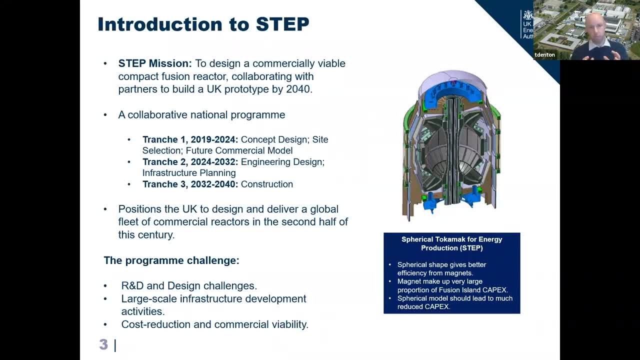 needs to be inherently a collaborative programme. I don't believe, as I look at the UK industry, the global industry, that there's anyone who can do this on their own. Now, whether that's in a supply chain mechanism, a collaboration mechanism, partnerships we're going to need. 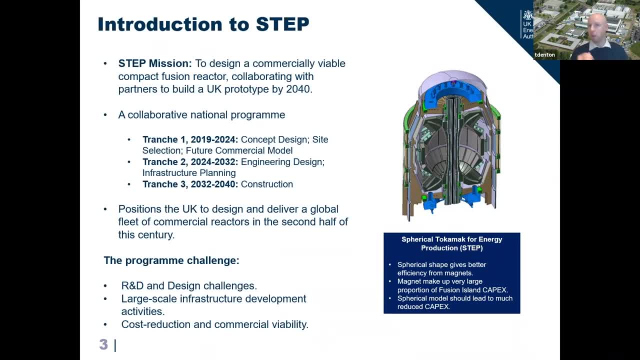 to work with others throughout this programme, Be they in academia, supply chain, innovative sectors, established sectors. this will always be a collaborative endeavour And that will extend once we come to the infrastructure side of things- I'll talk more on that in a moment. That will extend to working with 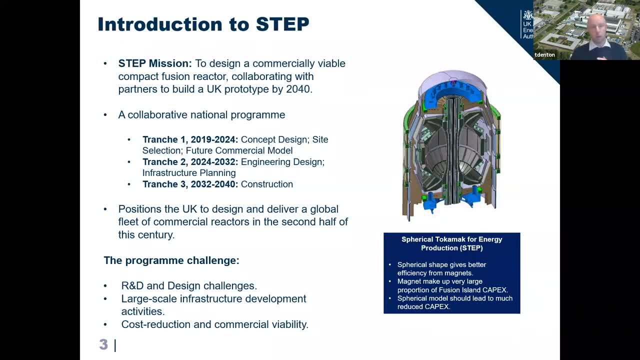 our host communities, communities all over the country, and engaging them in that exciting, challenging vision of bringing forward the programme. The programme is structured in three tranches, as is traditional for programmes of this scale. In these first five years, we're very focused on bringing forward a concept design undertaking. 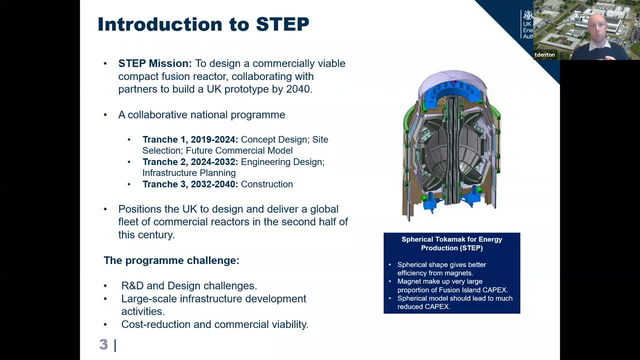 a site selection where we will build the tokamak and looking at the future model of the programme. In tranche two we expect to deliver the full engineering design of that and, of course, deliver the swathe of infrastructure planning activities that I'll say more about in just 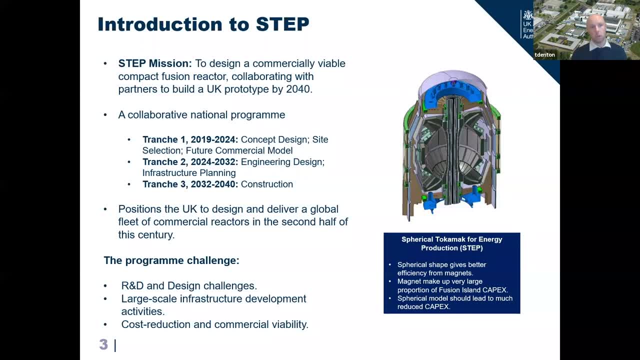 a moment to enable us, in 2032, to bring in a construction phase that will see the step machine completed by 2040.. 21 years- 21 years, I think, can seem like a long time. Of course it can seem like a long time It. 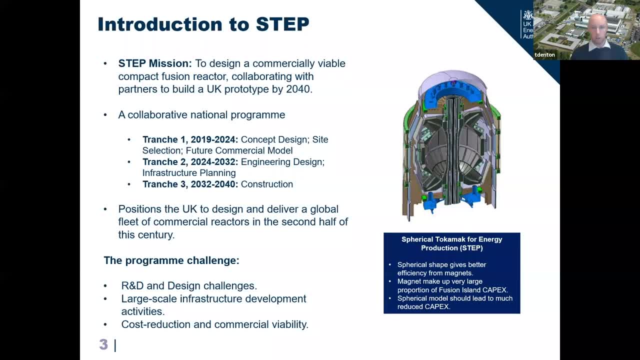 is a long time in any of our lives, But in infrastructure terms this is a tight, concise schedule. We have to make sure we focus, we bring forward work as far as we can and we deliver the programme in the right way for the right cost, on schedule. And if we do, 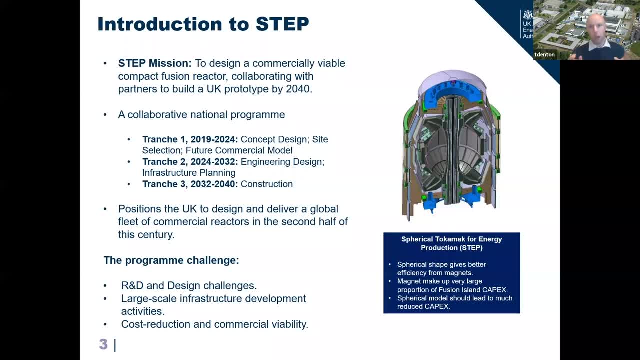 that, if we achieve our goal, it positions the UK- not just UKA- the UK- to design and deliver a global fleet of commercial reactors. We are in this transition and we should do that in the second half of this century. 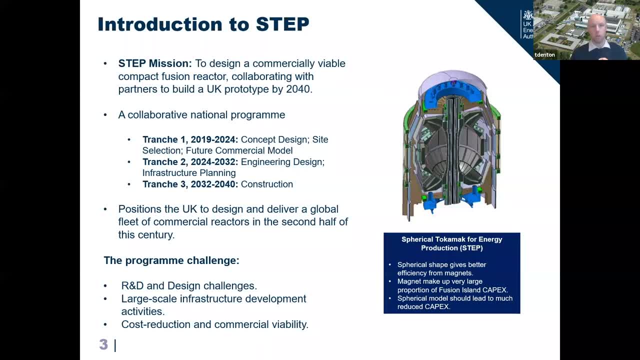 I'll talk a bit more in a moment about policy drivers for that and for fusion to play a role in not just a global electricity mix, but in a global energy mix. Now I say all this like it's easy. Of course, there are huge, huge challenges we must overcome. 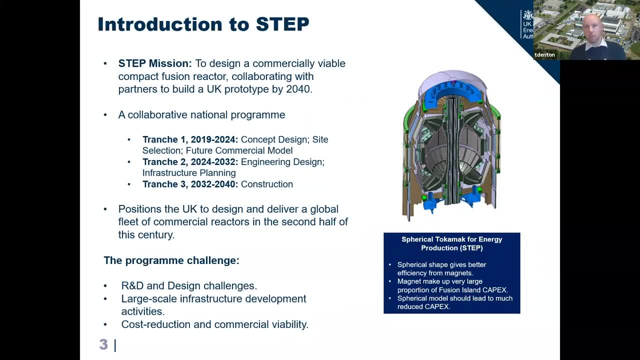 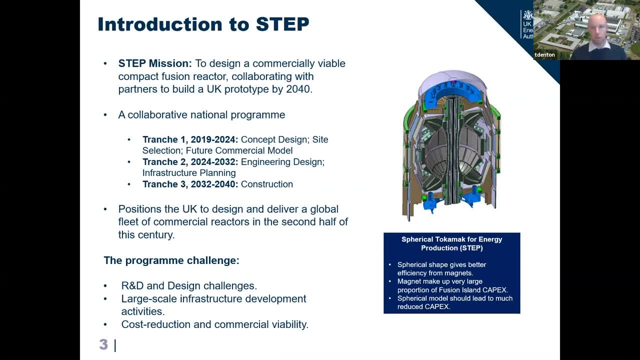 we'd already be doing it. There are serious R&D and design challenges that we must overcome. Indeed, the programme is about overcoming those and bringing forward this product to market. Alongside all those, there's large-scale infrastructure development activities, Even with known, proven, well-understood technologies, delivering nationally significant. 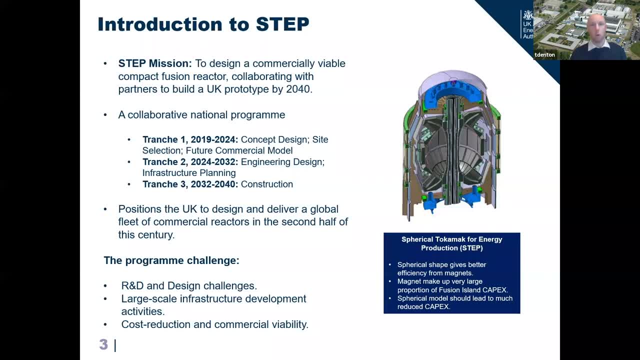 infrastructure projects is costly and brings all sorts of challenges and risks with it. We need to undertake those as we design the product And, of course, cost reduction. commercial viability: We want to bring this product to market at the right point in the right way. 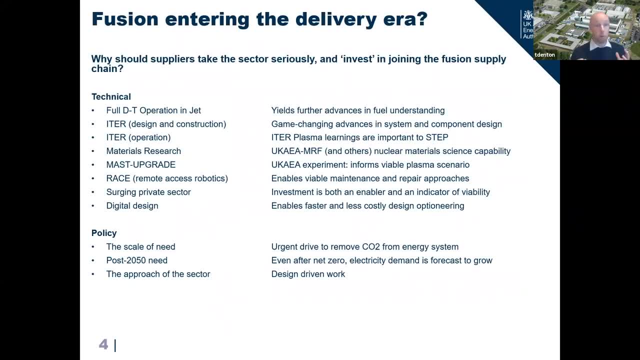 I want to share a slide here which we in fact wrote talking to supply chain a while ago, talking to suppliers about how exciting the fusion sector was. I'm sure there's a couple of supply chain colleagues on this call now. One of the great things about this meeting, in fact, was 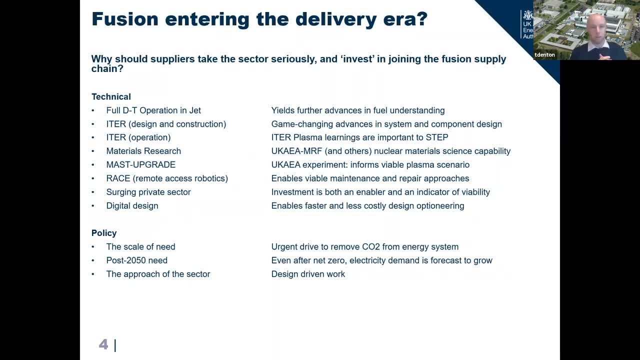 seeing the breadth of people who could attend And the suppliers asked me: well, why should we take the risk? Why should we focus our slim business development resource on you, on fusion, on STEP, Why should we take you seriously? And my answer is in this list of bullet points that I'm not. 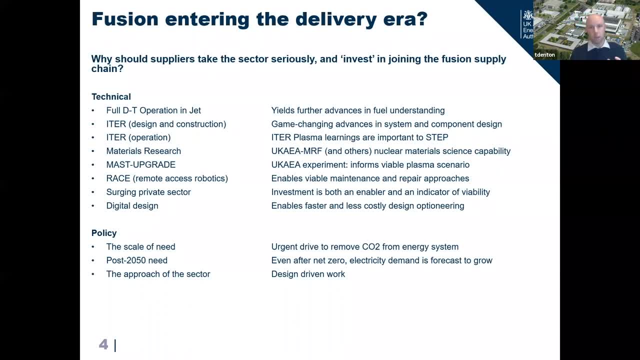 going to go through one by one but, I think, show the credibility of the sector of the technology. But piece by piece, challenge by challenge, this sector has proven its viability. It's getting increasingly close to showing that we can bring forward the products which we need to bring. 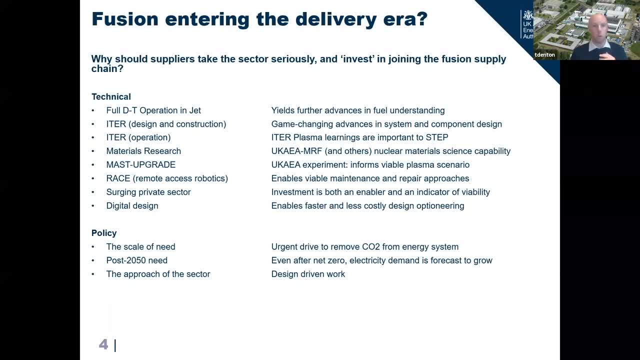 forward, Whether that's in the work we've done on MAST, whether that's the work that's been done globally to bring forward ITER, whether that's remote access in race materials, research, digital design. all of these factors enable success And in doing that, they enable credibility. 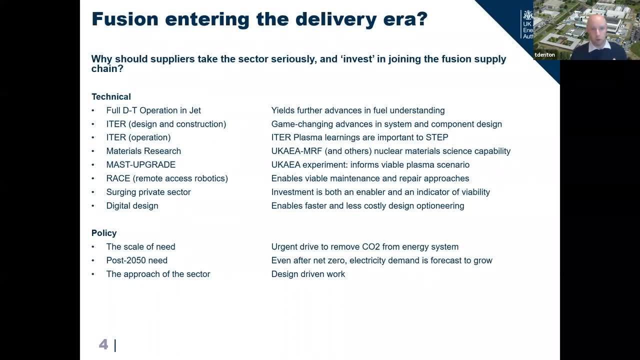 to our program. So look at digital design, for example. It's far faster, far easier, far less costly to model designs now than it would have been 20,, 25 years ago. That's material change. We need to look also, of course, at policy. 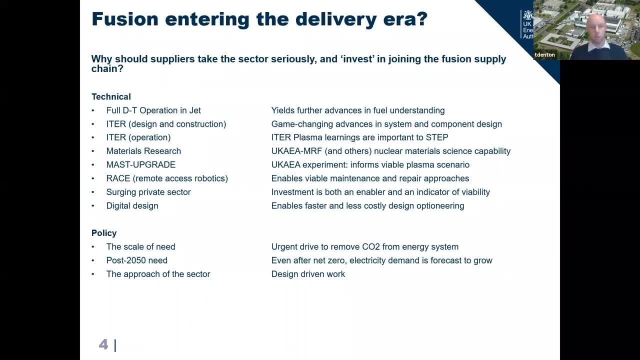 the scale of need to remove carbon from our global economy. I don't think this has ever been clearer and I don't think it needs me to say very much more on it now. I think the old phrase- or that old, in fact, but the well-trodden phrase- of act as if your house is on fire because it is. 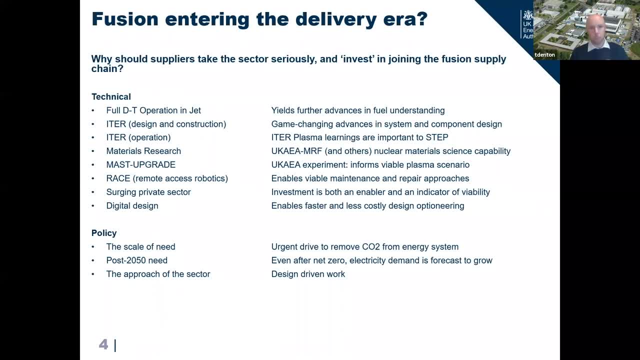 sums that up better than I could. We have to look at the post-2050 need as well. Net zero is a critical goal, But net zero doesn't sustain unless we keep bringing forward low-carbon technologies. As global living standards rise, global energy demand rises and potentially electricity as a 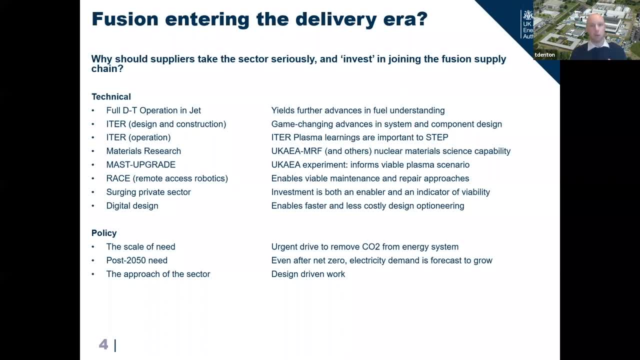 proportion of energy rises. we will need secure, stable, reliable supplies in the second half of this century for low-carbon energy and electricity, And I believe this is where fusion has a vital role. And, of course, the approach of the sector, the increasing focus on design-driven work. 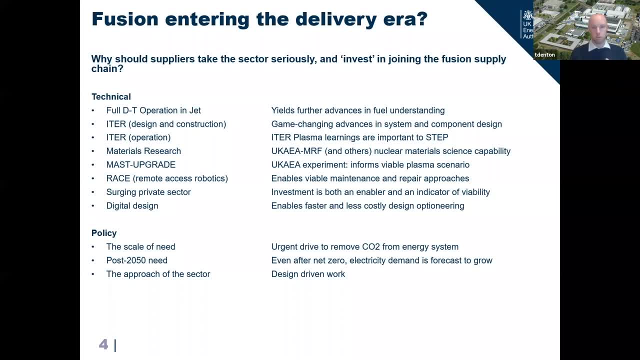 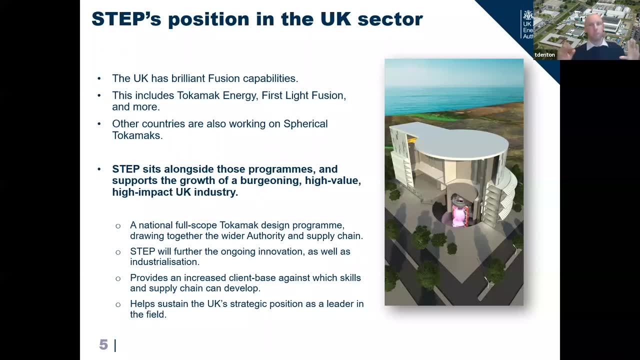 moving from R&D toward delivery. And look, I want to just sort of step back from our own program here and reflect for a moment that STEP is by no means alone. STEP is not the project that does this. This STEP is one of a number of very, very important projects And the UK has wonderful. 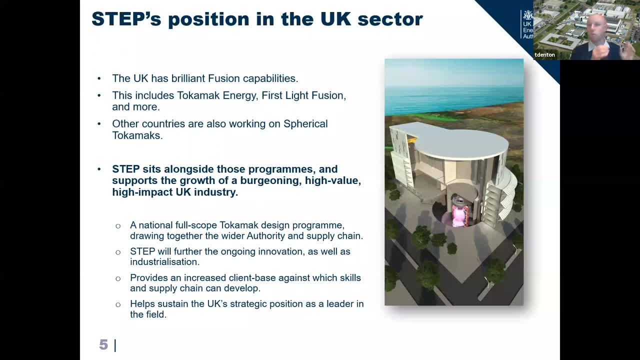 fusion capabilities. You look at Tokamak Energy. you look at First Light Fusion. you look right across the supply chain. You look at the British contribution to ITER, which is incredible. The UK has a strong, capable and vibrant industry which is going to be vital to supporting us. 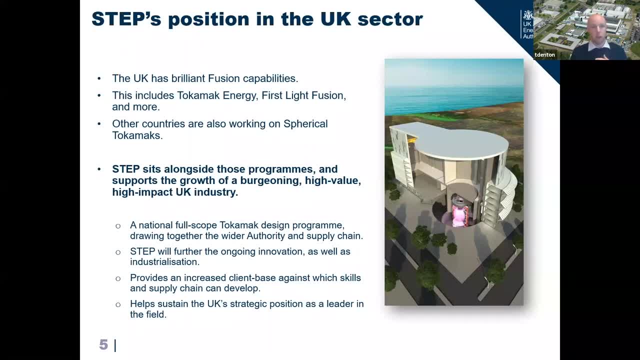 and it's going to be vital to delivering wider projects, And there are other countries working on spherical Tokamaks as well as a range of collaborative international programs on fusion. STEP sits alongside these programs And in doing so we support the growth of a burgeoning. 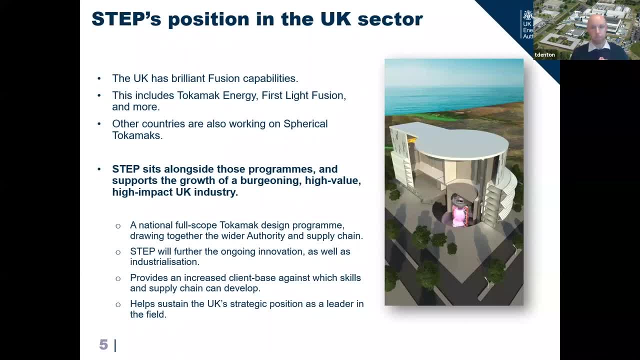 high-value, high-impact UK industry In what way, We believe, a national, full-scope Tokamak design, that is to say, a green Colorado-based, unparalleled international enterprise, but also a developing enterprise. We believe it is a real way forward for us in our business. 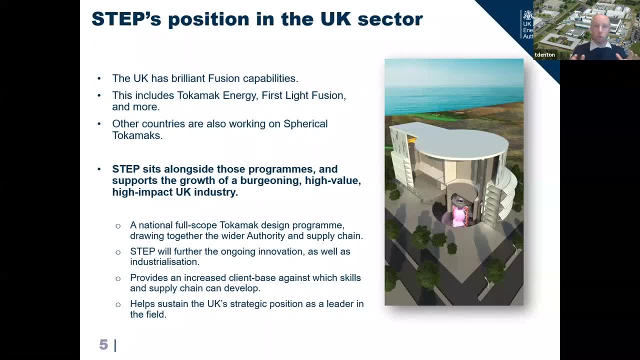 For example, we do it for a purpose. We have a part-time job as a service provider and we're very, very, very lucky to be part of that. We also see this issue happening not only at the ЕCA, but as a result of the 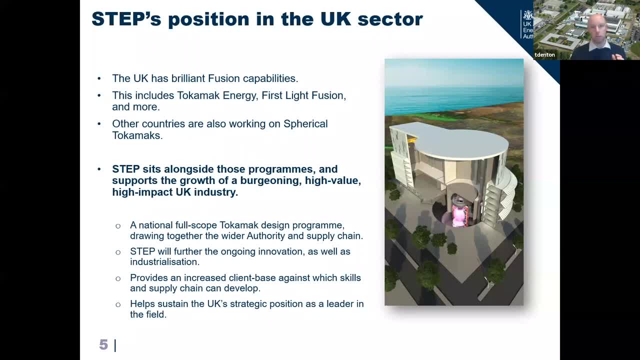 sustainability provisional waste reduction programme And, just to add, it's something that we are charged for as well. We're charged for the services that we provide to the UK, And this is what we mean when we talk about going from an R&D to delivery-focused sector. 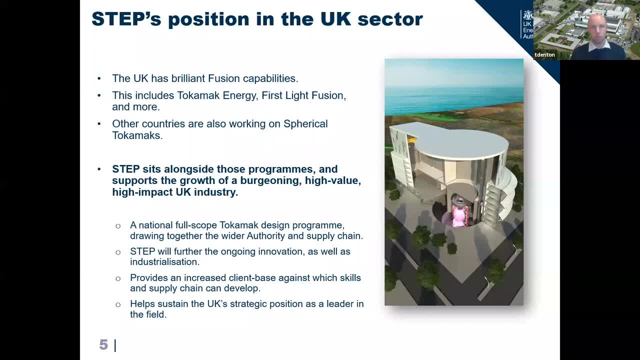 That's not to downplay the challenges that remain. I've been clear on those and I won't say anything against them. but we have to focus on that journey from the lab to the street. Step third is ongoing innovation as well as industrialisation in the sector. 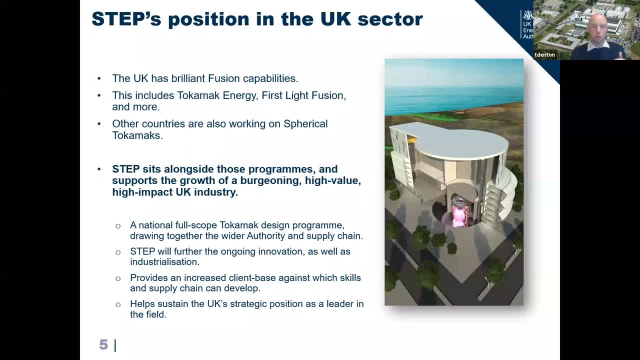 And I think importantly again, if the supplier is on this call, STEP provides an increased client base against which skills and supply chain can be developed. It allows the sector and the industry to grow confident. they've got multiple clients, multiple opportunities. 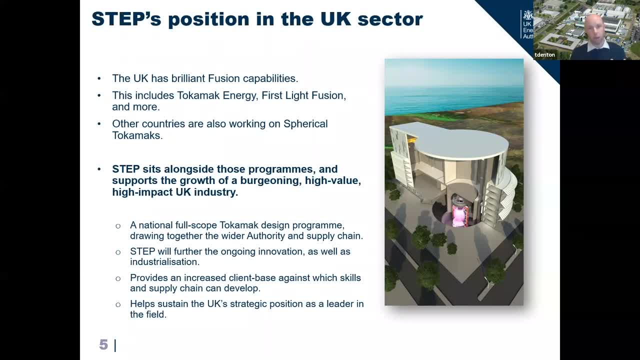 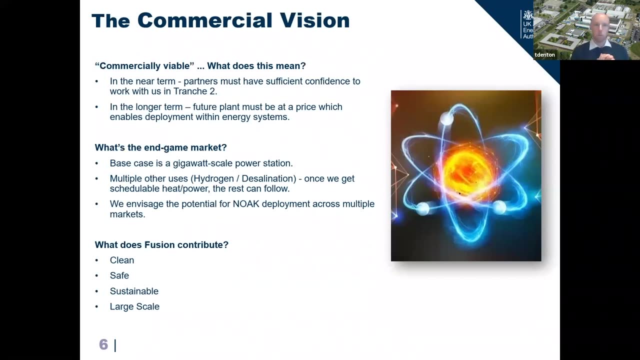 It provides that basis, that business case for growth of a private sector in the UK and beyond. And, of course, STEP helps sustain the UK's strategic position as a leader in the field. Commercial vision: what does commercially viable mean? Well, look, I'm really clear on this. I think we need to be credible. 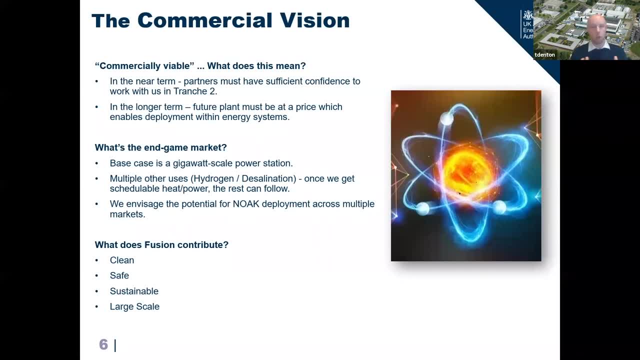 And we need to partner to have sufficient confidence to work with us in Tranche 2 and beyond. We need to be an attractive prospect to suppliers, to partners, to collaborators And, in the longer term, future plant must come to market at a price point which enables deployment within energy systems. 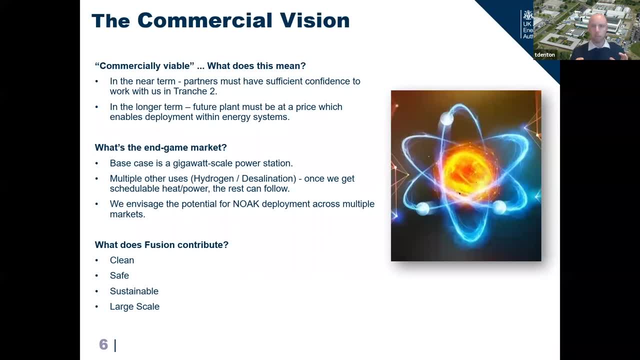 Just as I was kicking off, I noticed a question landing in the Q&A about: do you believe fusion could ever break even? I think we have to believe fusion can break even. I think we have to be committed to realising that Because if we don't, the country, the region, the world is going to face the challenges of global climate change and the need for energy supplies without this fantastic tool. 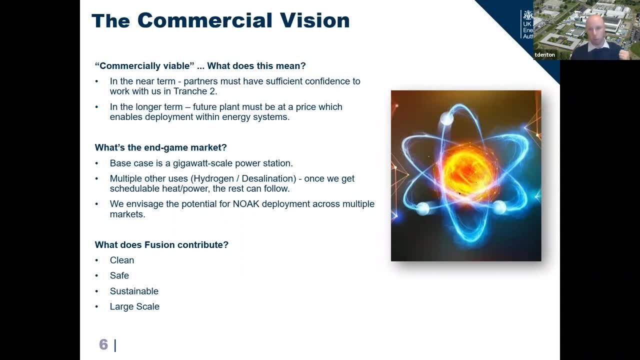 If we can't bring that reality forward, we cannot put this tool in the toolbox to take on the challenges we all face. What's the endgame market? We're quite open. Yes, of course, a gigawatt scale power station is one brilliant option of what you can do with this. 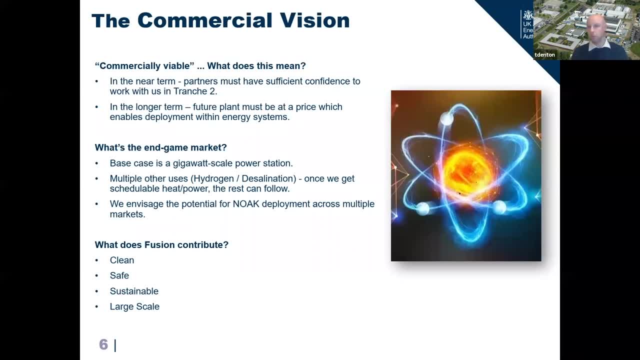 But you shouldn't forget the other uses: Hydrogen Desalination, District heating, Many, many things. We need to understand them, We need to explore them, We need to look at what our product could provide to customers and to people. 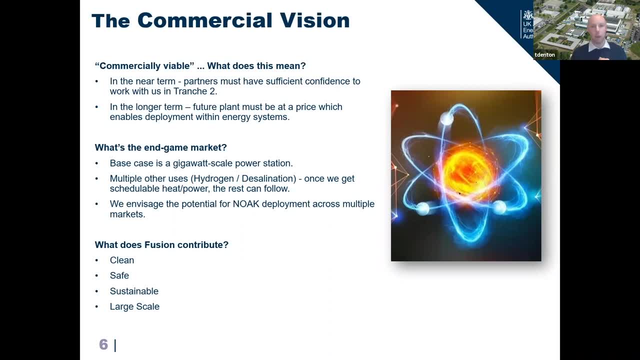 Colleagues in the authority use a fantastic phrase when they talk about schedulable heat and power. We need schedulable heat and power. When I worked in fission, we used to talk about our power plant as kettles. It's a very complicated kettle. 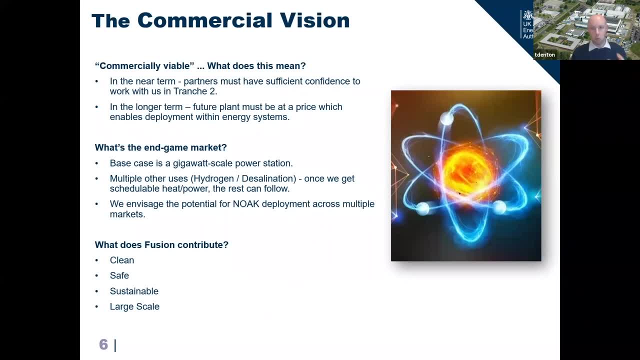 It's a kettle with, in that case, very high risk, But it needs to produce steam in a reliable, controlled, predictable way, And that steam can spin a turbine or produce a range of other uses. We envisage a phrase- I've used a horrible phrase here that colleagues can sneer at me- for later. 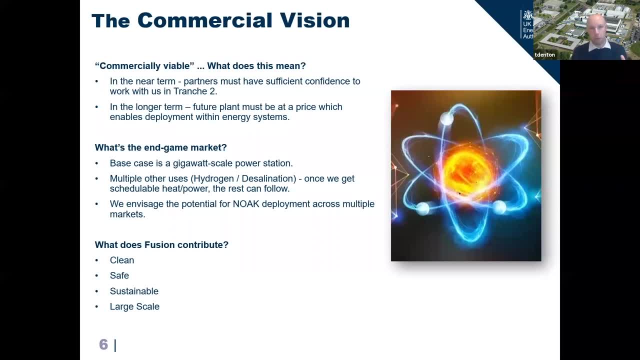 Nth for kind NOAC. This is when you have a fleet approach, multiple power stations coming off, Each one bringing efficiencies, learnings, improvements, enhancements, Going into multiple markets for multiple uses. And, of course, what does fusion contribute? 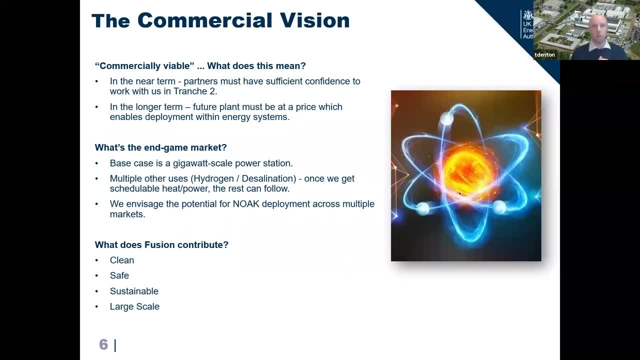 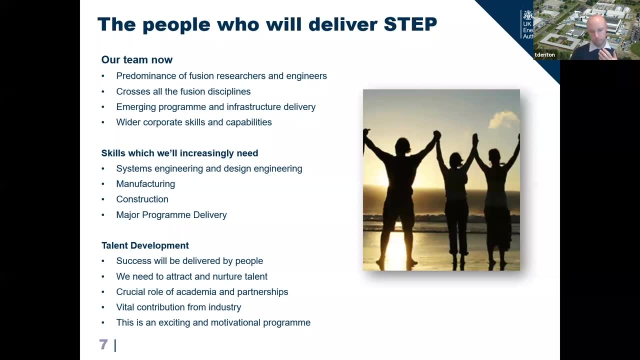 Clean, safe, sustainable, large scale power and energy. This slide means a lot to me, And it's one that I was talking to colleagues about yesterday evening as we looked to bring this presentation together: People- Ultimately, all of what we're doing is about people. 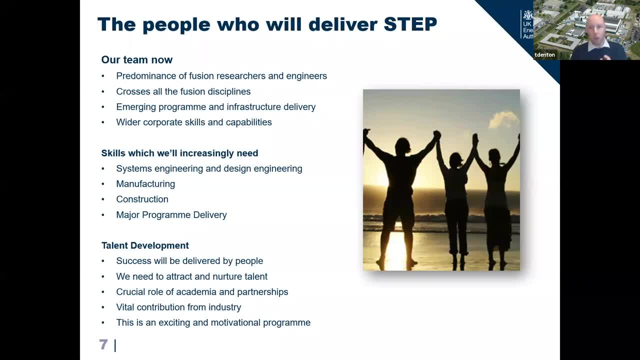 All of our success will be built on people. Anything we get wrong might well be because we don't get the right people. Our team now has a predominance of fusion researchers and engineers. rightly so, because it's a fusion research and design engineering task across- right across- the fusion discipline. 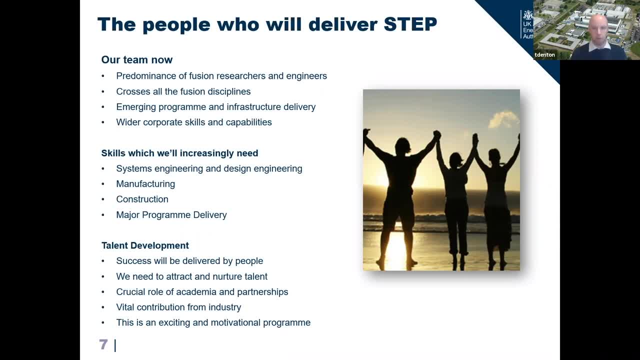 One of the exciting things about being at UKAA is that breadth of knowledge, the breadth of capability we can draw on. we can reach into as a program and get experts in their fields to help us understand and overcome these challenges. We've also got an emerging program and infrastructure delivery capability we need to develop. 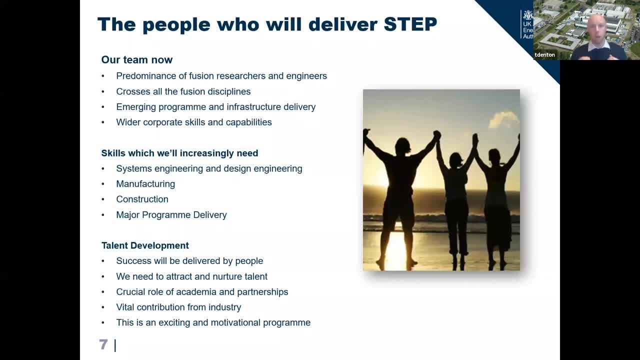 This is not just about designing a product, It's about bringing a program forward And, of course, the far wider set of corporate skills and capabilities which we need to run, administer and deliver a program on this scale. Skills will increasingly need. I mean I've grabbed four here because I could have flooded 10 slides with skills we'll need. 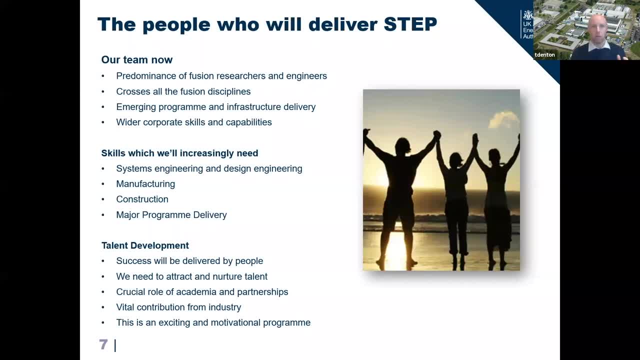 But systems and design, engineering, Manufacturing. There's no point designing something if it can't be made Construction. We will need to build, to plan, to build and to build at the right cost this plant And, of course, major program delivery. 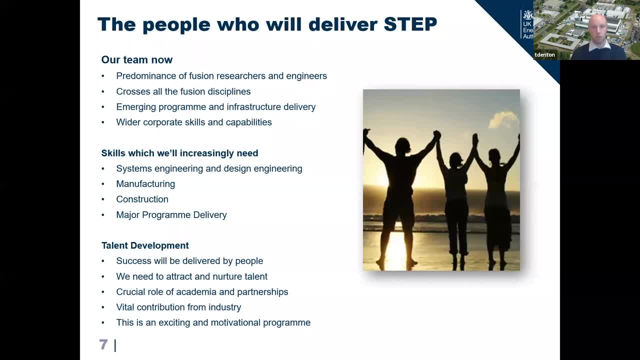 Bringing together commissions, consents, regulatory consents, supply chain, skills, capabilities, our own work to bring forward a project where we design, permission, build and then operate this facility: Talent development. Success will be delivered by people. We need to attract and nurture talent. 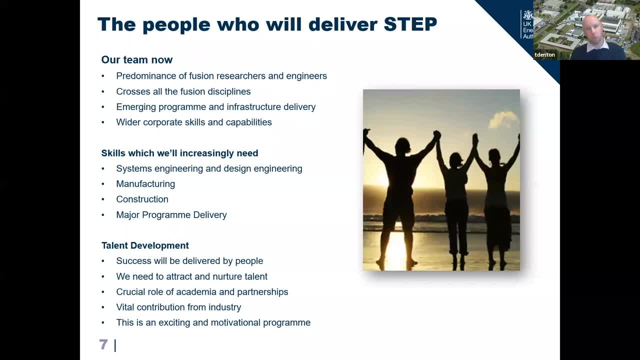 There's a crucial role in that for academia and partnerships and a vital contribution from industry. All the talent on the program does not need to be in the authority. We're already working with wonderful suppliers across the country and beyond To help us by bringing niche expertise or bringing capacity. 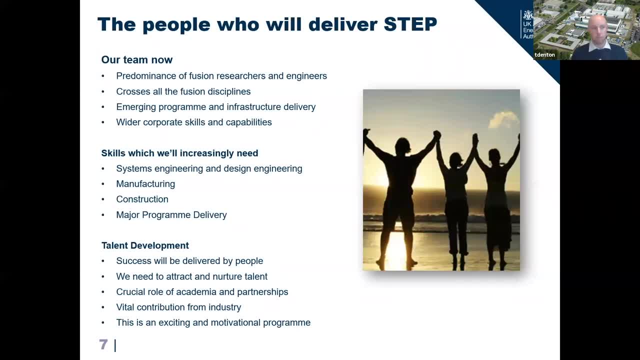 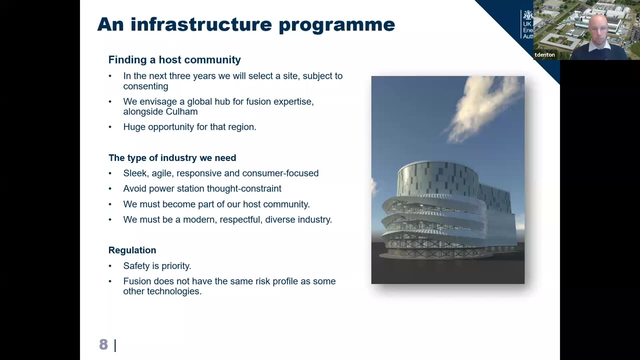 All of those roles are vital to our success. This is an exciting motivational program. We really do hope to bring that to bear, As we put together the team on which success will be built. The infrastructure program I've mentioned here is a real challenge. 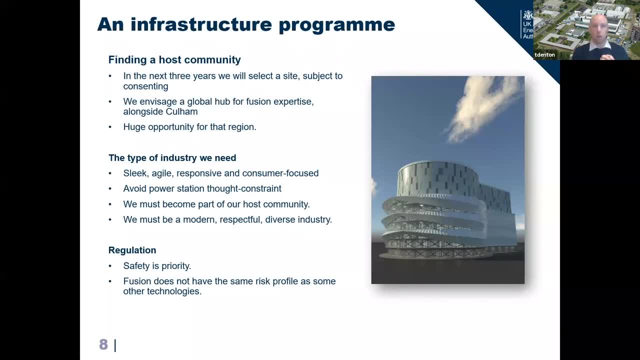 And of course we need to focus on that. We need to find a host community. In the next three years or so, we expect to select the site for STEP, clearly subject to consenting. It should be very clear. This would likely go through a national consenting regime and everything will depend on permissions. 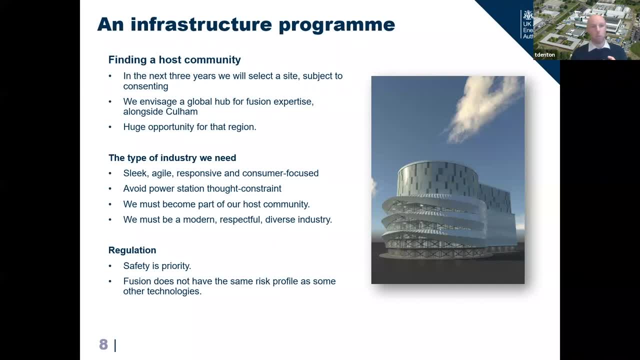 We hope to pick well, We hope to make that site- and that's like we have visited- a global hub for fusion expertise, just like Cullum. This industry, this sector could have a phenomenal impact. I'll talk a moment in a moment about that. 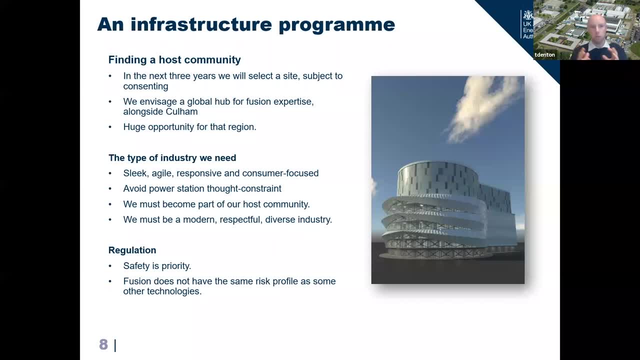 And we believe that building a hub of capability around our site and around Cullum will enable that The type of industry we need to grow. we need to be sleek, agile, responsive, customer focused. We can't get locked in an idea of what we think is best. 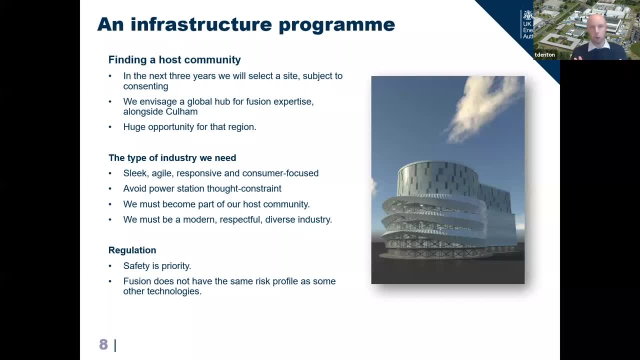 We have to deliver something based- the phrase we use in industry is stakeholder requirements. What is required of this product, What is required of this program? to be successful, We need to avoid thought constraint. We need to start here with an open mind, be completely up to speed with the best practice, the best understandings, how to optimize the design and then the delivery of energy infrastructure. 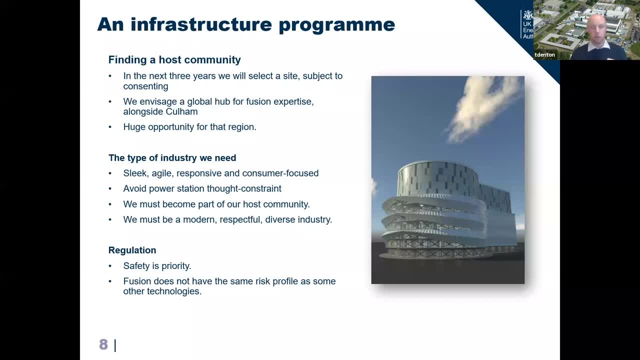 We need to become part of our host community, completely part Um. anyone who's worked In big industrial sites within a community understands that you can't sit there and just be a good neighbor. You have to be instinctively and fundamentally part of that community. 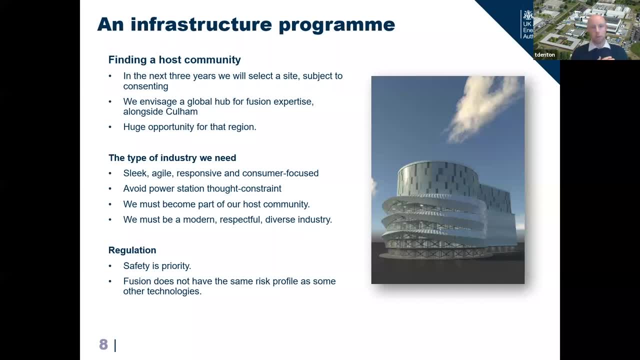 That will be essential for step one that matters a great deal to me. We must be a modern, respectful, diverse industry. We need to access the best talent we can from every sector of society. Bring that together. We need to value diversity of thought, diversity of ideas, because this is the way in which we're going to crack the big challenges. 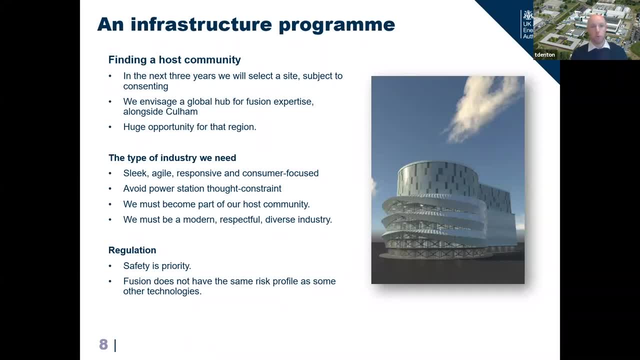 We need to value diversity of thought, diversity of ideas, because this is the way in which we're going to crack the big challenges that we'll face. And, of course, regulation safety as a priority. It must always be, But we have to recognize if using doesn't have the same risk profile. 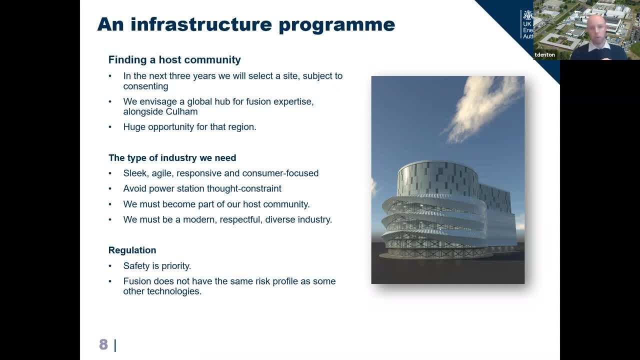 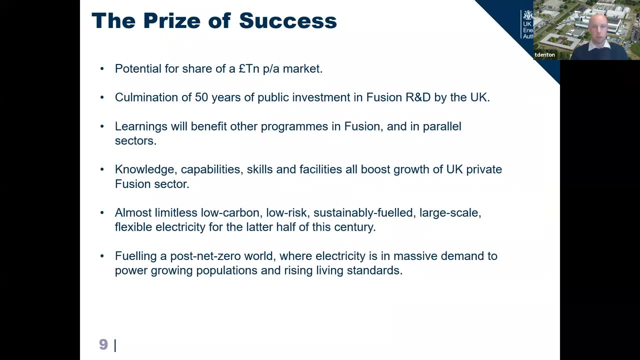 Many other technologies and things need to be proportionate to that Prize of success: Potential share for the UK, Multi trillion pound market Culmination of fifty years, plus a public investment in fusion by the uk and elsewhere. we believe our learnings will benefit other programs in fusion and in. 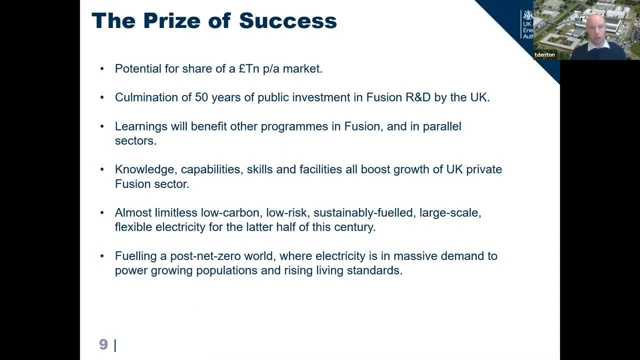 parallel sectors. we want to see spillover benefits. we want to see the understandings we develop help the energy sector and beyond. we want the knowledge capabilities, skills and facilities that we build to boost the growth in the uk of the private sector and the public fusion endeavor. 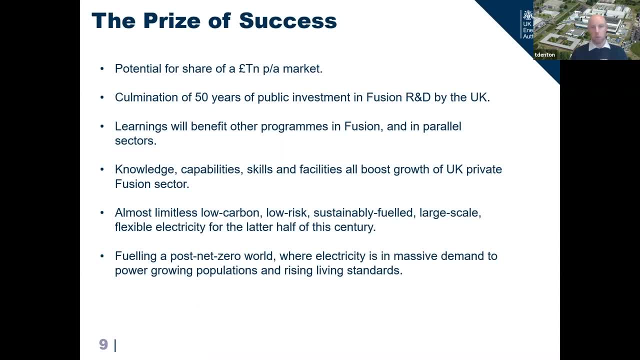 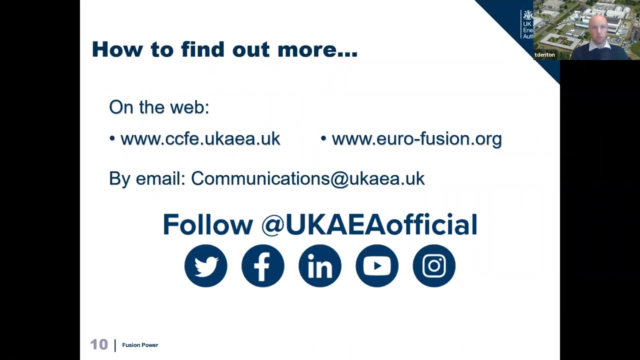 and of course, we want almost limitless low carbon, low risk, sustainably fueled, large scale, flexible electricity and energy for the latter half of this century. i said i talked for 20 minutes. i think i've talked for about 23- a number of ways to contact us there. i'm going to leave that on the screen. 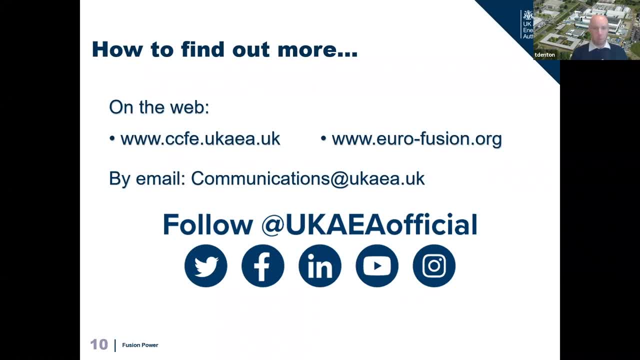 and with that i'm going to stop talking. i'm going to open the q a and we can have a real discussion. now this is where it gets clunky people. i'm opening q a boxes and i'm trying to read them, work out the answers and 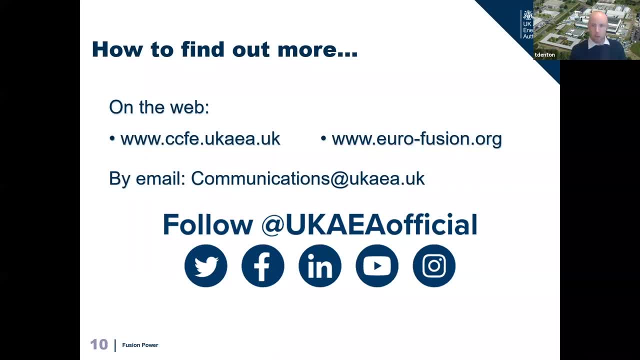 talk to you all in one day. so please do forgive me if things are a little rough around the edges. i've got my post-it notes so i can think as i go. so let, working through the q a top to bottom, do we think that tokamak can reach the break even? yeah, as i say, i think we have to show that we can. 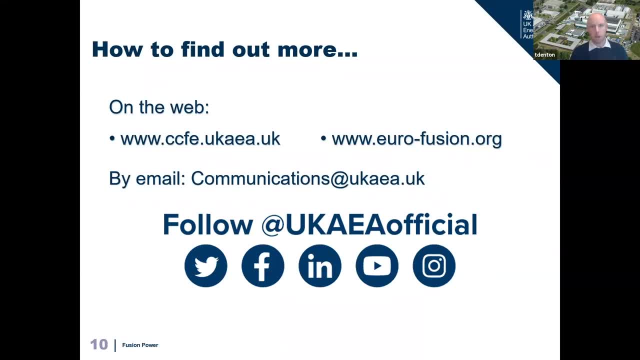 i think that's the challenge we as a program face um, and it's not just about breaking even. it's about being a commercially desirable product. it's designing a product that fits the right market need and bringing that product forward in the right way, and i think that's the challenge. 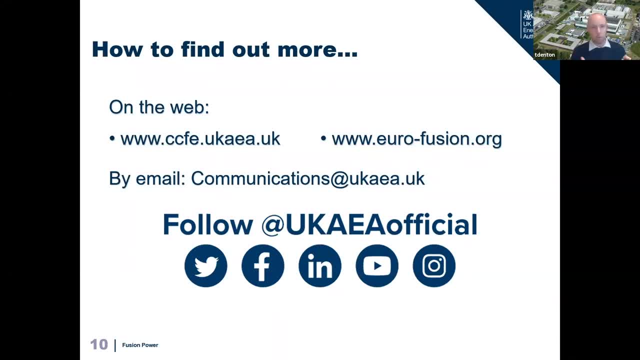 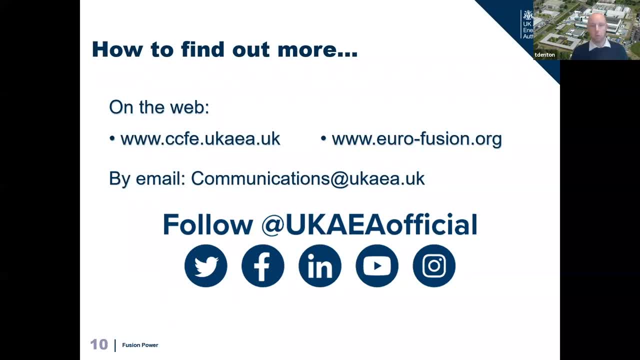 pausing there and talking to my colleagues from uk. i don't know if you're able to remove questions i've answered as i've answered them, um, or if you need me to do that, but uh, if you can, that would be great. next question: do you use magnetic, cold, confined plasma and spherical tokamak? 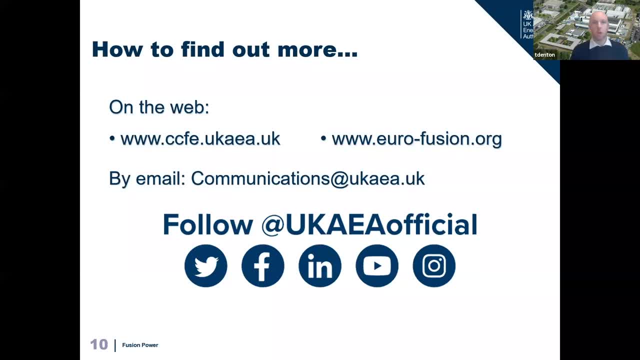 radiation tokamak can be done. what can you do? okay? so look, as i say at the start of this, i, my degree is not in engineering. um, of course, the the concept of spherical tokamak is not wildly different from that of a conventional tokamak. we believe, uh, the ratio could give us a better. 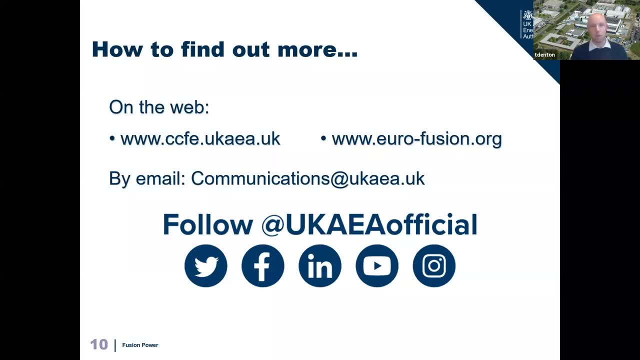 solution and that's why we're exploring that. but of course it's a magnetic based system to confine the plasma. it's just as you'd have an eta or in jet. um, yeah, you're right, the cost of magnets are extremely significant. we need to make sure we're getting the right. 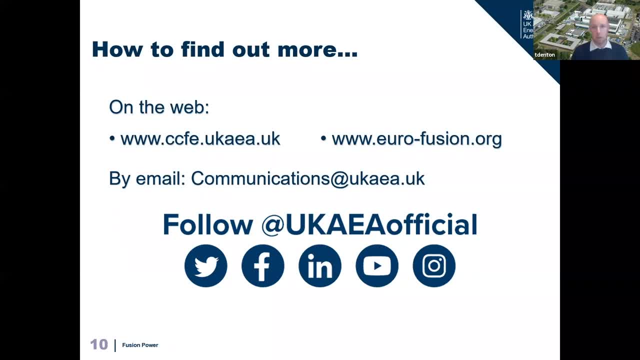 designs sourced in the right way, from the right type of industry, with the right materials, um, and that we increase the longevity of those, those items, as far as we can. you know, anything inside a tokamak is going to suffer really significant neutron exposure and that's why. 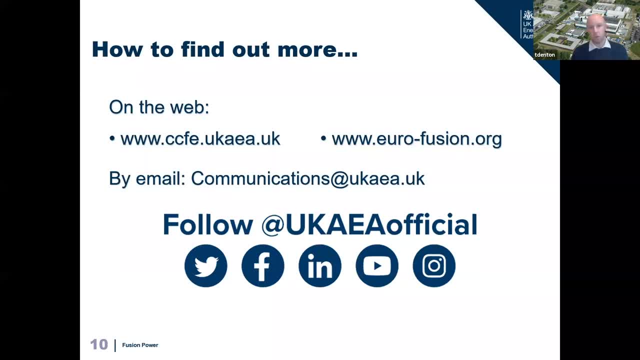 we need to make sure that those internal components, those in vessel components, not just magnets but beyond- have the longest lifespan they can um a to reduce the, the proportionate uh, so capital cost, but also to increase the lifespan, thereby increasing your time between operational outages and also reducing, as far as we can, the amount of material we have to take out of the. 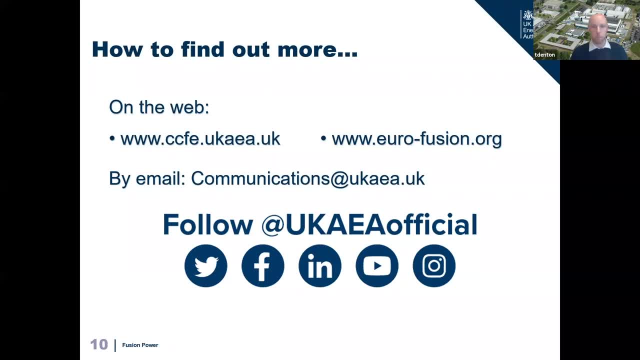 mac, um after use. next one on how much com between um, uk, uksa and esa: fusion energy with game changer with respect to man space, um, yeah, you know what? i've got a colleague who was super knowledgeable about the potential space applications of fusion and i'm really sad he's not sitting here next to me. 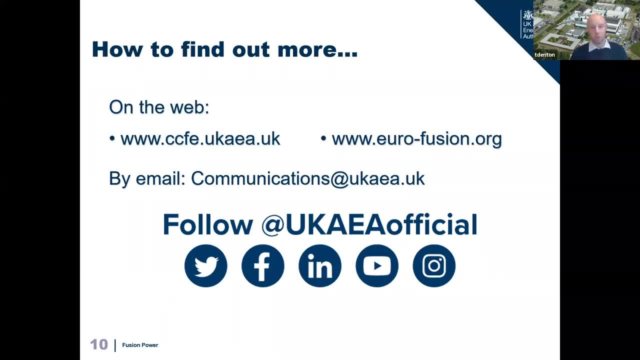 right now, partly because he's a great guy, uh, and partly just because he'd be able to answer that question. i know there have been overlaps between the uk and various space agencies. i can't give you the full detail of that, but if you hit the communications email address, i'm sure they can. 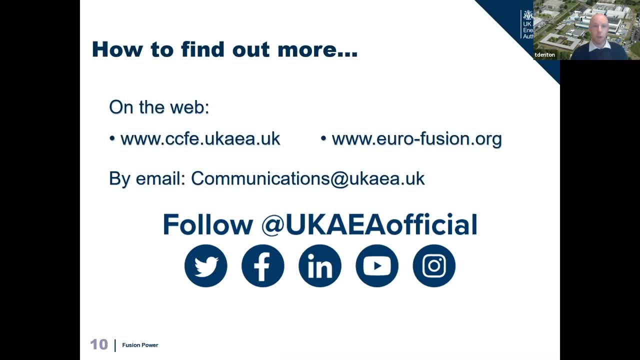 uh, share more. other companies have much more aggressive time scales. yeah, fair play. um, we understand that, you know we, we know that there's various time scales that the companies are working to and and really i wish them luck with those. um, we all want to see fusion come forward. what we've 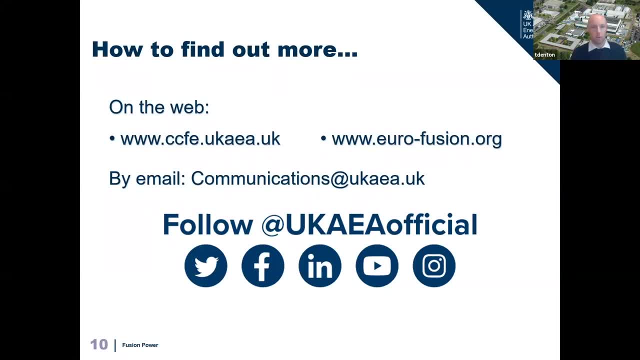 done in step is lay out a time scale and a program that we think we can deliver to meet our aims with our objectives and our funding levels. um, i think it would be disingenuous and unhelpful if i were to sort of start talking about steps. i know we need to compete, we need to be first, we need to. 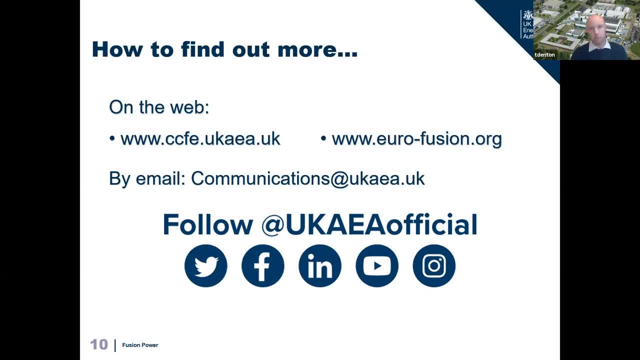 be this: what we need to do to show the credibility of the technology to our audiences is to deliver a strong, capable program to the fastest time frame we believe is credible. as it stands, we believe that's bringing forward a prototype in 2040. of course, if breakthroughs enable that to be accelerated, that would be great. 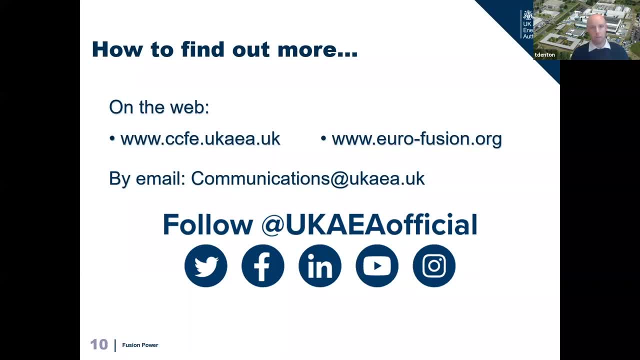 um, but we're really focused on on delivering that, that, that time frame um which is going to be, you know, in itself a significant piece of work. um, it'll be interesting your thoughts on going from master user size st to step size st in one step versus having intermediate devices. great question. 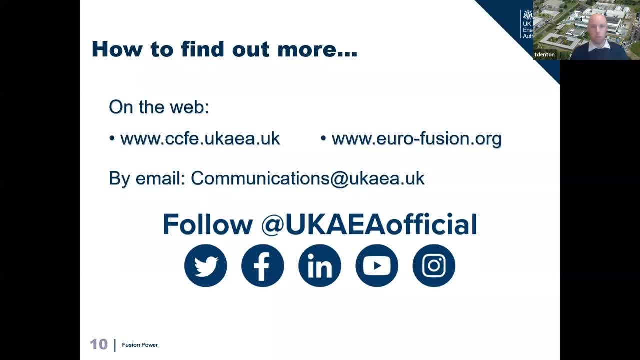 any step considering a high field approach. um, seems like i feel like some juice capex, so i can certainly answer the first one straight up. look, you're dead right. you know, any big, difficult sort of first of a kind or nearly first of a kind uh program has options you can. you can prototype to. 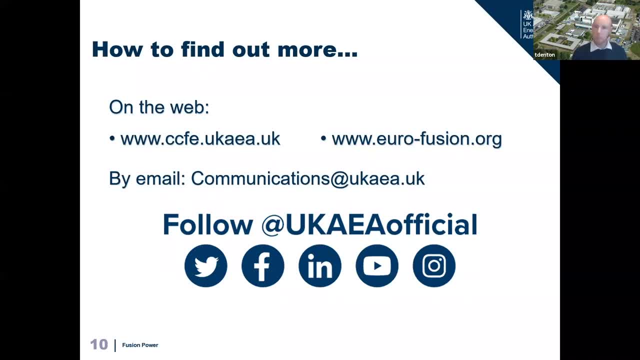 the nth degree. you can keep on prototyping. you can take small incremental steps. every one of those incremental steps takes time, takes money, takes investment, takes consenting, takes permissions, takes delivery, um. or you can look to take bigger steps, um, and in doing so you you potentially get a much bigger 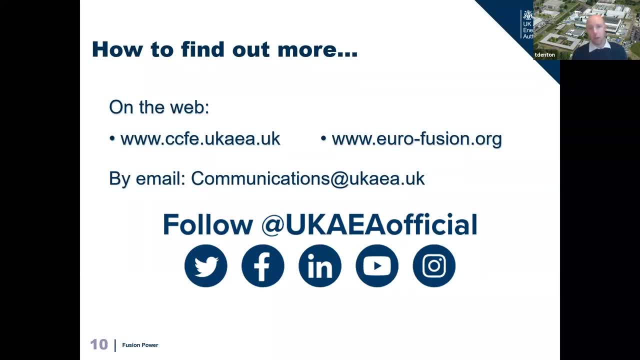 gain, but you have a much possibly bigger challenge along the way. we believe that in this country we've got some, some really significant knowledge based on, on, obviously, first, jet operations, but also master. you is in the st space, um, and that is right and enables us to move towards a step plant um. 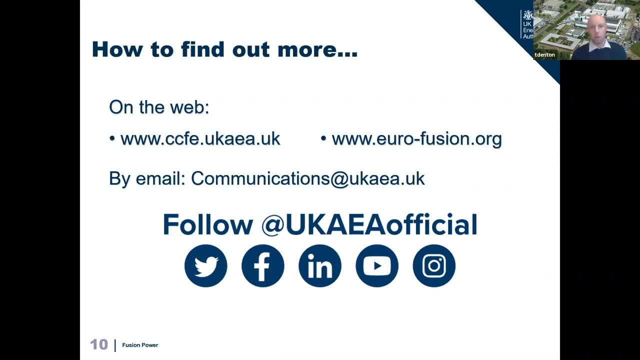 step prototype plant in the right way. um now, i think we should be clear that that what we're not proposing to do is to bring forward the perfect, final, best ever spherical tokamak that's going to produce loads of predictable energy in that first go. that's why, in our mission, we talk about building. 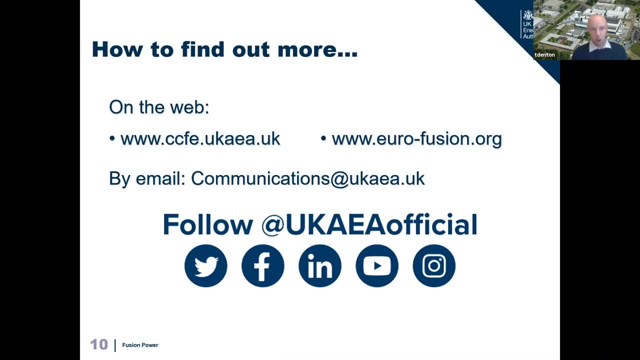 a prototype, um, but we do think it's the right ambition and the right aspiration at this stage of technology maturity, uh, and at this stage of policy need. regarding the point on high field approach, um, look, candidly, i can't give you an answer to that. i'm sure we as a program can, uh. 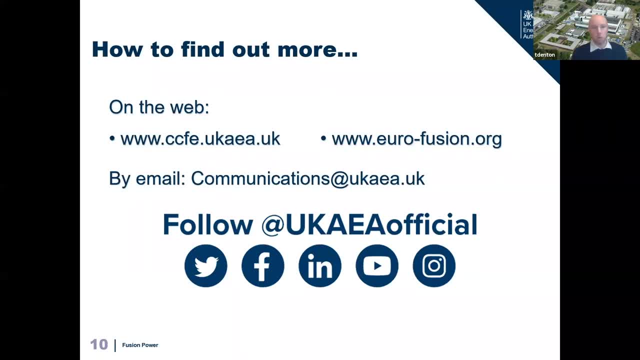 and again. um, i don't think we can see your contact details in the box, but if you want to pop that into the comms email address question, we'll get you an answer. what are the criteria under consideration for the host of step? this is a really interesting one and i i'd urge colleagues- and in fact there's another one there on citing 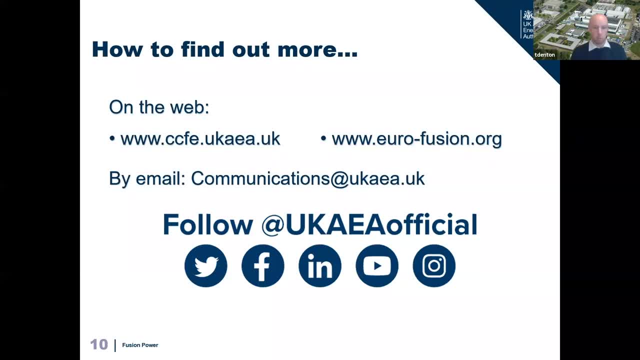 policy. so let me just say we will be publishing um protests by which we expect to select a site in the not too distant future. of course, the selection of site will be a matter for secretary of state. what we need to do is provide a recommendation for the site to be selected in the 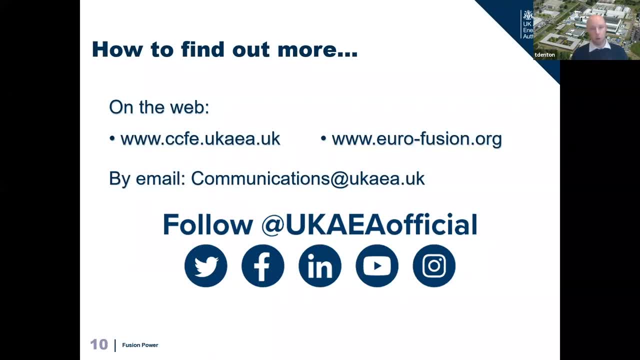 um to the sos um throughout this first part of of tranche one, the criteria, you know. we'll publish the full detail in that process. i don't want to dive into that too much now, um, but if you look at it, there's, there's a whole host of criteria. that will be the same if we're building a football. 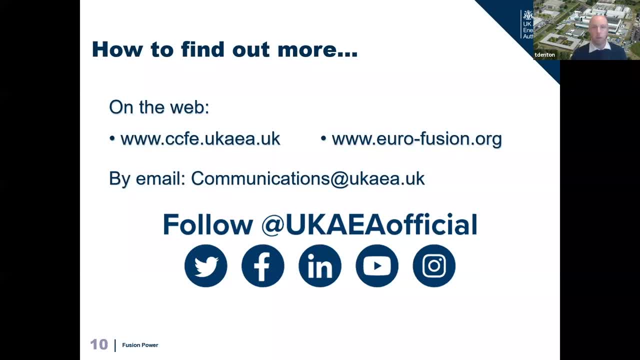 stadium or a train station or a- you know- water plant, in that you need the right size of site, um you need the right access criteria. you need the right seismology, um you need the right broader capabilities. you need the right industry locally, um you want links to academia and these things. 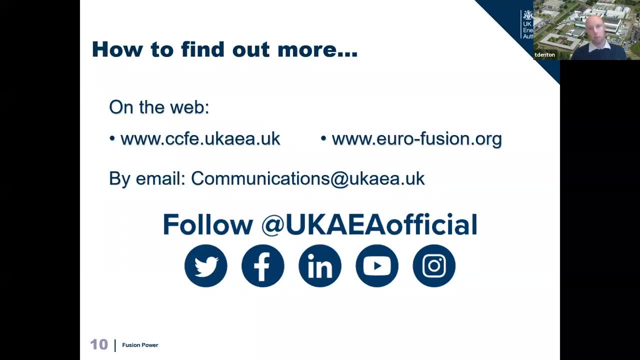 are fairly standard across the infrastructure. there's a lot of learning from best practice we've done there. then there's a number of more power station specific criteria um, such as water and grid connections, which would reduce the the challenges we'd have in designing um the plant. 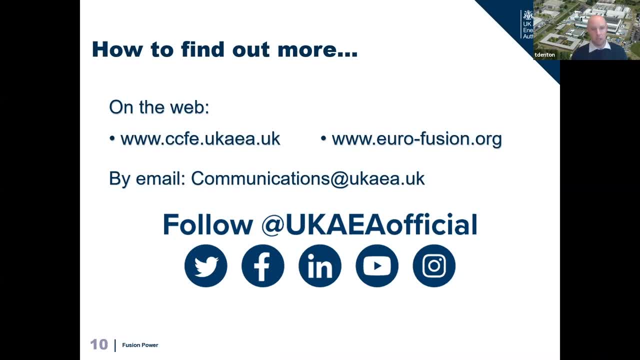 but look, all i can say more on that is: we'll publish full details fairly soon, um which they'll be fully in the public domain um as well. q a on that, uh, and it'll be a very, very open and allowing perspective challenge. um will might be able to be a little bit longer as well, but 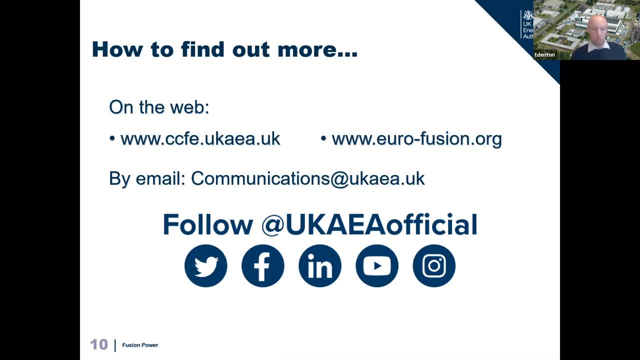 i'm not going to go into too much detail about some of the the the impact that it's going to have, because the community is going to be a bit longer and we're still looking at a variety of ways of um how to deal with and how to deal with them to support the outside data that we can use. so 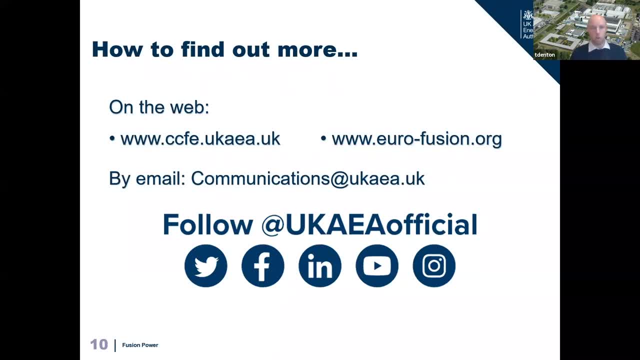 um, we're moving to the next phase, so we're going to reflect on that. i don't want to close on the nature of that, but i do want to reflect on that and talk about how we know what the potential is for our butpolitik, but also what we do know about what we're doing and how we're making the. 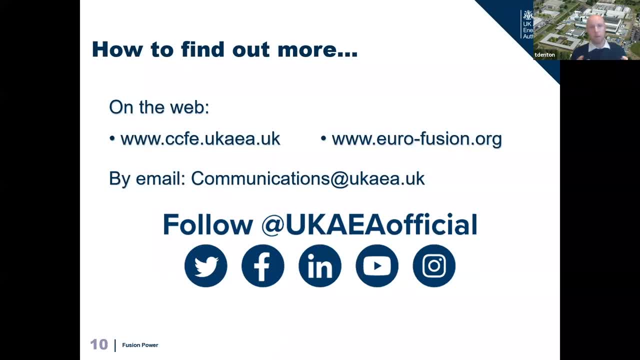 decisions and what we're taking on. it's going to be a very valuable part of that for us. as a technical colleagues briefed me on, is the um, the magnetic field of the potential efficiency rating you can get from your magnetics. it's something we think is potentially very interesting. we'll 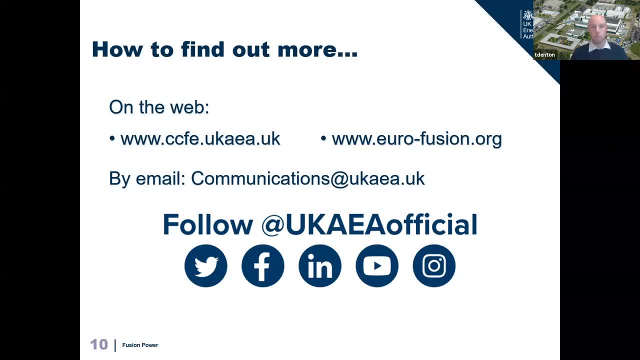 explore with mast. we want to explore more um with step, but of course, look, you know, this sector is going to explore a lot of technologies, and rightly so. um we as a country and authority, still very closely involved with eta, which is a conventional tokamak, um i think they also have. 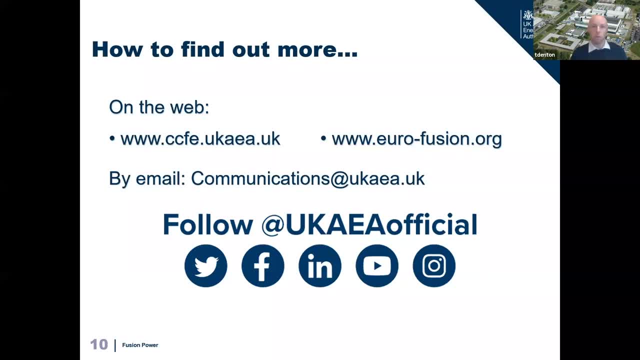 a number of very, very, uh, important capabilities. you know, i think, when you're in early stage industry, anyone who sits there and says, oh no, we can completely close this down and answer the question now. here's the only solution. frankly, that would be a little naive. um, the first one. 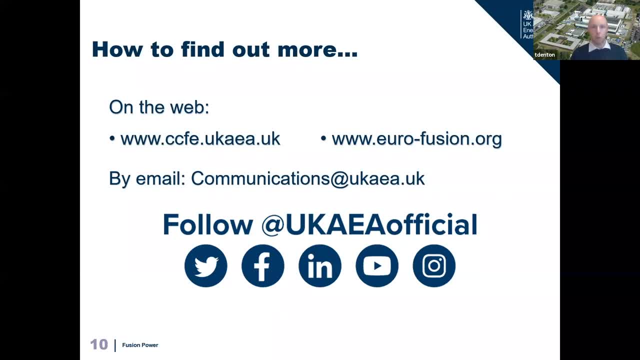 and the first few will be expensive to build. i think you're right. um, all the investment we needed for it to start delivering returns. uh, a big sticking point for efficient parts of the uk how it pay for step. should government pay for it, private enterprise or what? 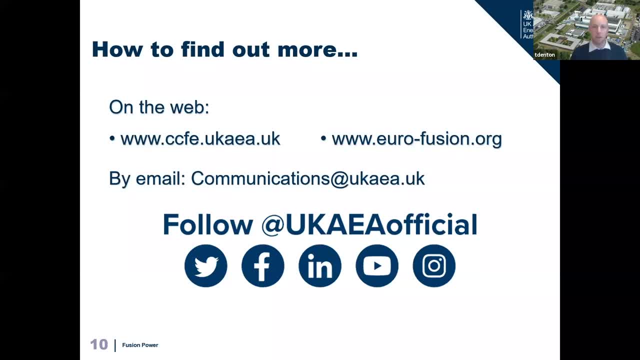 um, yes, i think that question boils down to: can i answer the entire financing question in one go? now, probably can't go that far. look, yes, big infrastructure is expensive, without a doubt, big infrastructure is incredibly expensive. um the return on investment and the value can be incredibly good. um, what kind of challenge can be is quantifying um and capturing. 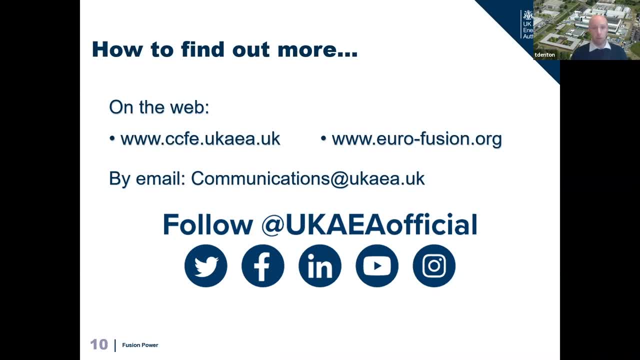 that at the early stage, when you're seeking that finance- and yeah, you're absolutely right that the efficient plant at the gigawatt scale in the in the uk have struggled to secure the level of financing we need- how will it play for step? i mean, there's a number of things we are working to design with a cost conscience. you know this is. 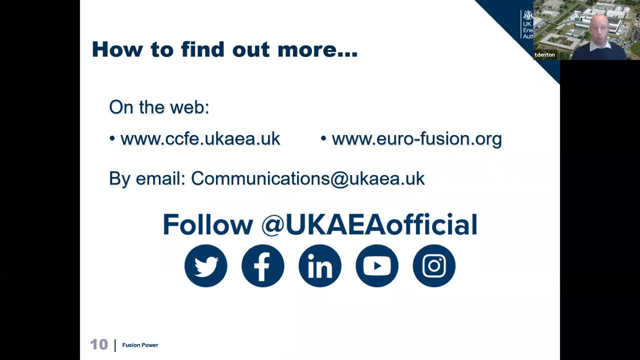 not a bring forward product at any cost type of program. this is bring forward the right product which is the right thing for the right market at the right cost program. so the first point on any financing question has to be getting that cost in at the right point. um, in terms of the route between, 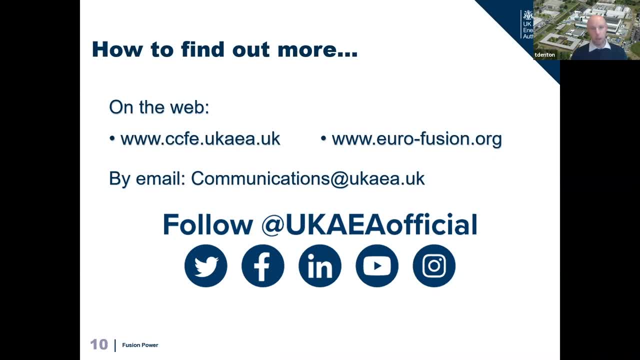 public and commercial financing. clearly, it's going to be a very interesting area to explore. the government plays a front and center role in this program at the moment, and we've been clear that the government remains vital and, of course, an increasingly commercial aspect of the program is important too. um, honestly, i think trying to define the exact breakdown at this stage of 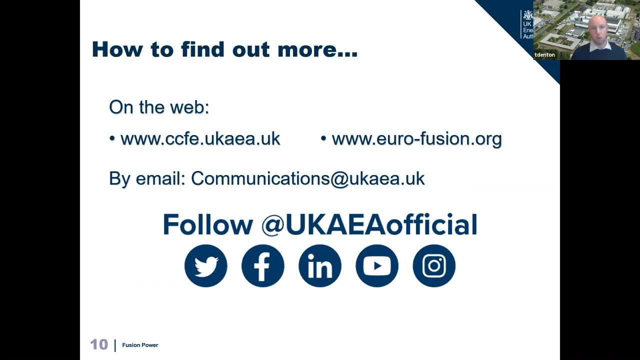 technology maturity and program maturity would be ambitious. we've got to focus right now on designing the tokamak. um is step using. it's very important to be able to design the tokamak with conventional uh low temperatures magnets or hds magnets. um, sorry for the technical question. 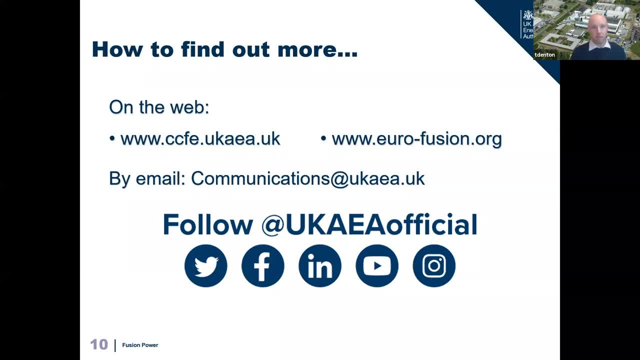 thank you, someone's very understanding there. no, look, um, we've not yet made a magnet technology decision. we're exploring a number of magnet options. uh, the sort of the chief engineer on step said to me: i think it's probably within my first week on this program. he said to me 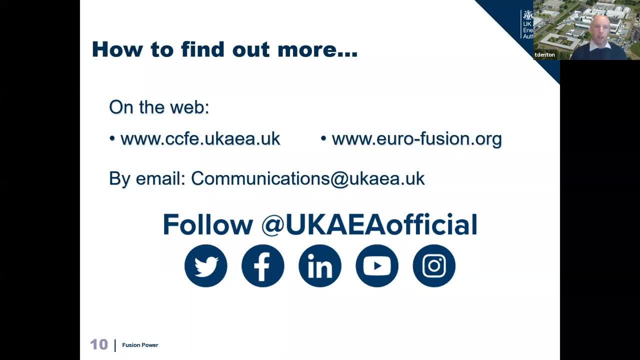 look, the thing with fusion is you change one thing, you change everything. um, and that's something that's been really interesting for me to watch as we've gone through the program, and i think it's something that's been really interesting for me to watch as we've gone through the program. 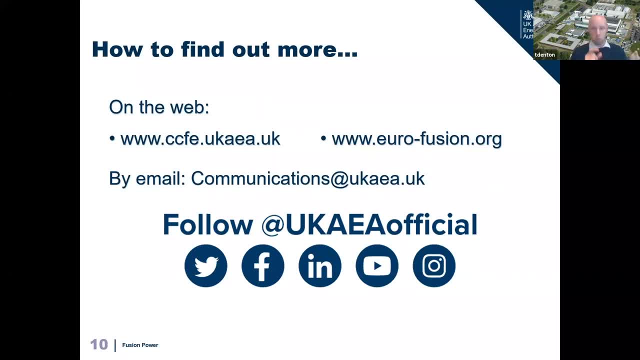 um that you know you can't start. this isn't duplo. you can't bolt together this bit and that bit. until you build a robot um, you need to look at the entire design of the robot um and understand what component parts you need. so there's a whole range of magnet technologies that could be. 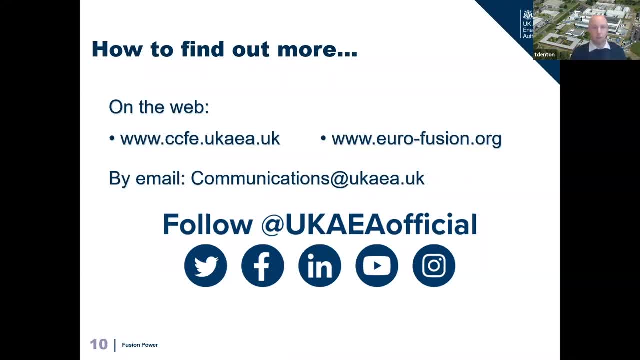 interesting. obviously, hts is an extremely exciting field just reading about it as a, as a lay audience, um, but it's not the only show in town and we need to. we need to work through those options and understand how they fit with the wider design. um, i know that sounds like a. 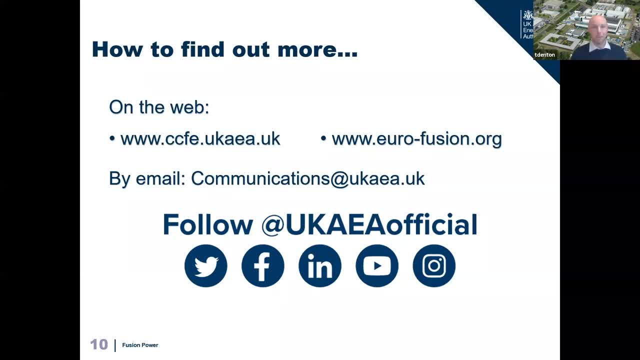 slightly political answer, but it really isn't. it's it, it's the truth as it stands. um, what are the engineering challenges to the success of step? really interesting that you've gone for the engineering challenges there and not the r&d challenges. i think that's a good, healthy sign for sector as a whole. 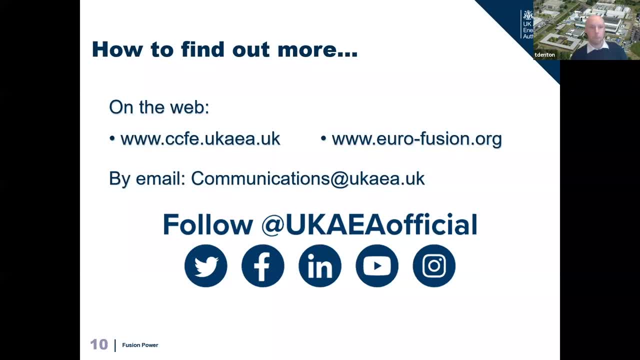 the key engineering challenge, of course, is integration. um, uh, we've got a number of design units and research units within the program, all highly capable, um, all staffed by some of the best in the business. the challenge is that we need to be able to do that, and i think that's a really 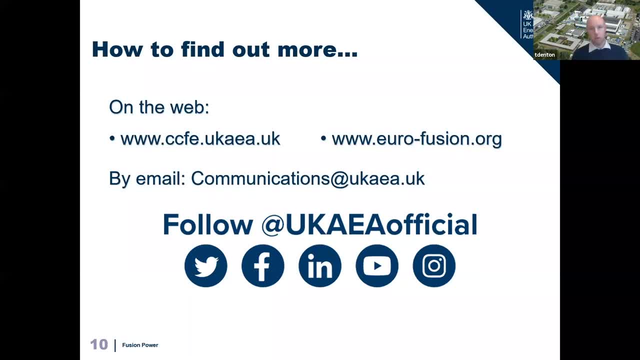 powerful idea that's taught by the government, and i think that's really important to be able to learn from them. um, i think that's a key, important part of the challenge is not to design a number of individual components. it's to define an integrated, effective system. um, and the more i study, uh, 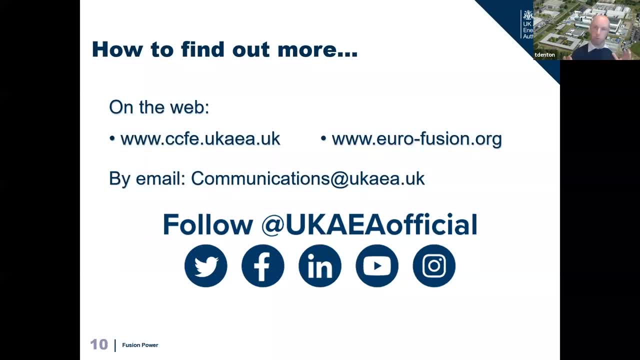 materials coming out of our integration team, our plant architectural integration verification team, the more it's very, very clear that the challenge is bringing all of these capabilities together that work with one another, um, and not having one or two sort of legs of the spider. they don't quite. 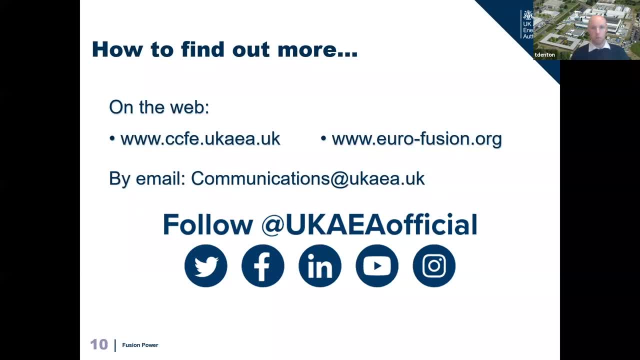 join up and one of the key areas where further research is needed to make steppe as its senior really interesting. i think there's- you know there's- a number of research areas that that we look at to make step a success. i think the other point is how can we research to advance? 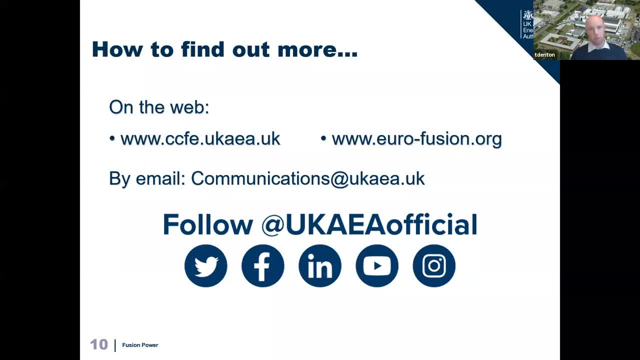 um the case of step, if you're looking at success, it's about understanding the right plasma model. you know, one of our great people describes plasma not as the show stopper but the show starter, and you have to bring that down. and of course, these things need design work and 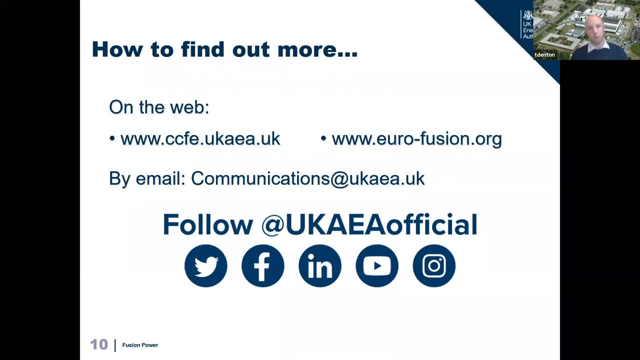 fundamental research to be viable? um and we hope to bring forward a number of of experiments in in physical form and in silico to to deliver that um 21 years sounds like a long time. is the road mechanism length? the tranches you described flexible if investment involvement is to increase? 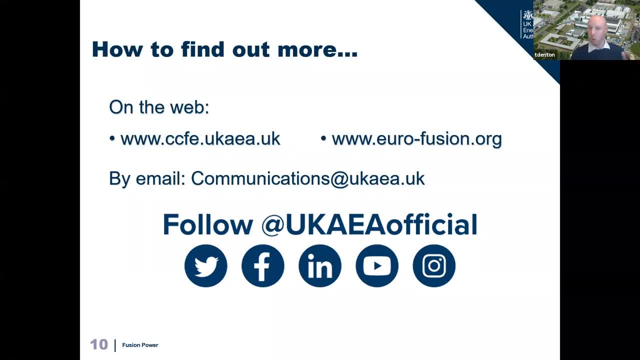 over the next decade. um, we see the time scales of project decreasing be offering. um, look, yeah, 21 years does sound like a long time and, of course, flexibility is important in a program. anyone this of this length, claiming they know the exact phasing perfectly and that they're not open. 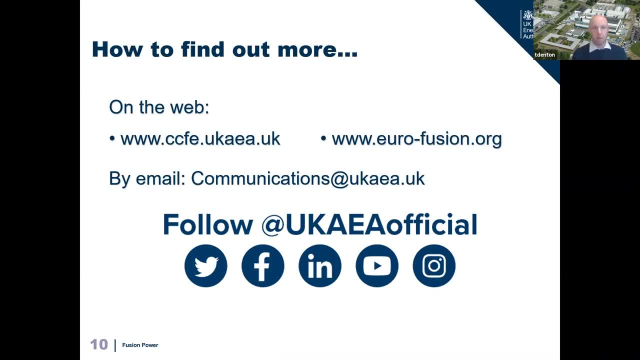 to new information. i think be um making a really, really interesting error. um, we have to be. it's a real balance. we have to be focused on the end point and driven and hold everything to schedule, whilst recognizing the need for, uh flexibility, um, in the way we do things, uh, and you know things. 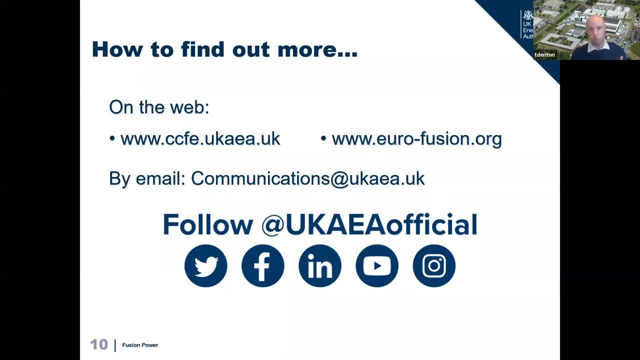 like tranches, programmatic mechanisms, program management mechanisms. of course, we have to be open-minded on what we need to look at, what the time frame was, what the investment looked like. the reality of these programs is, yes, in cases you can spend more and work faster, and in other parts of the program you have systematic constraints, be that the availability. 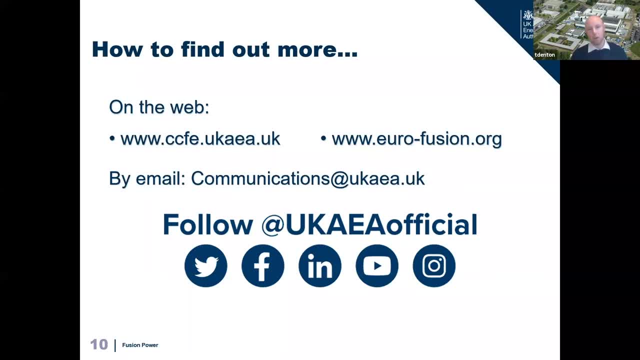 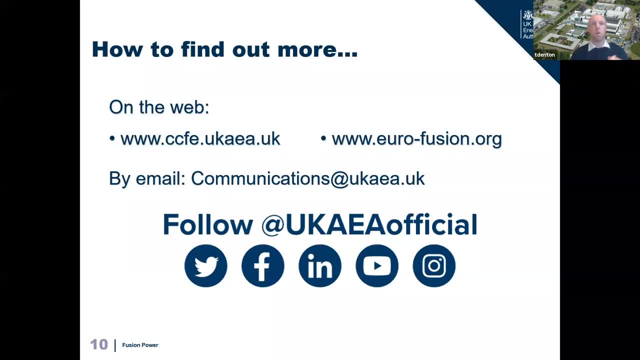 and you can look to accelerate. how can we join the program? brilliant question, best one today? um, look, there's a number of points here. um, individuals, we, you know, we recruit very significantly through our, our online portal. we advertise things very, very openly. um, i can't remember which of the more information points is best, but have a look at the website, i'm sure. 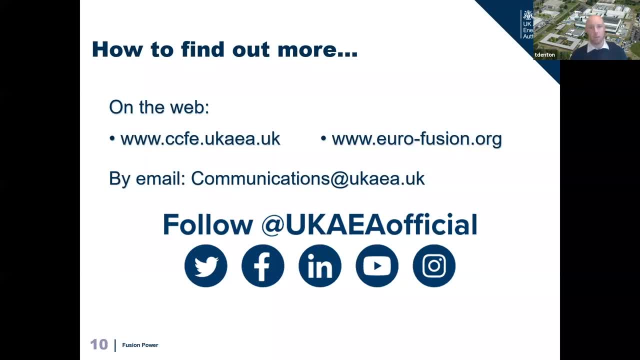 there's more there um. so, individuals, we're always looking for the right talented people, as i've said um. corporately, we have a very significant program of supply chain engagement, um, and we again, being a public sector body spending public money, we advertise our opportunities live on the step portal with the step procurement pipeline on govuk. um, so i really do hope there's. 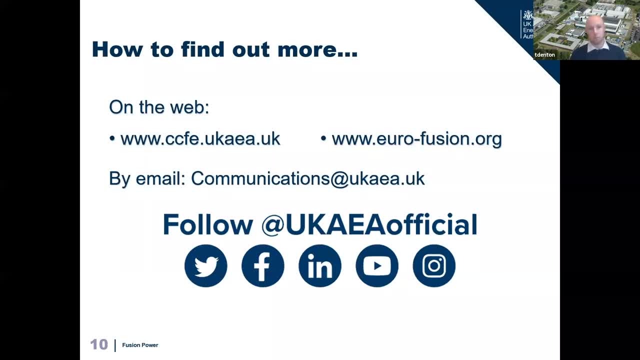 a couple of good routes there for individuals or companies to get involved. uh, what's the trajectory for industry becoming more involved broadly in the endeavor and at a larger scale? assuming by the endeavor you mean our program. um, we absolutely think we've. we've got a fairly high level of. 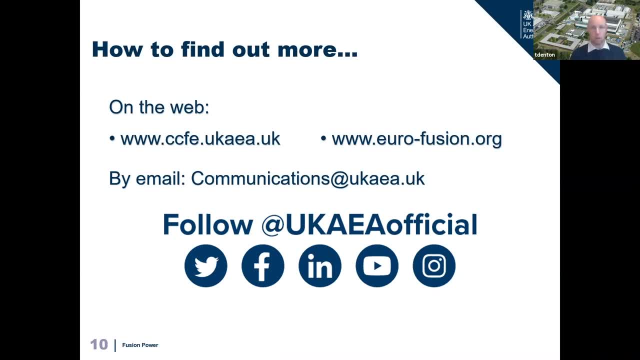 industry involvement. already, um, we've had a very significant number of- forgive me, the number's gone, but it's in the 70s- of companies who've worked with us just in the first year of program. i think it's about 79. um what we need to. 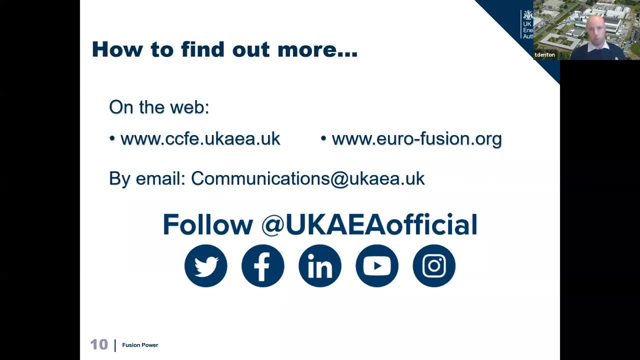 see, obviously is- is industry taking on bigger, bigger and modifying roles of that and i think you'll see that coming up naturally through our procurement pipeline, um, and then obviously, as we move into later tranches, there's going to be more and more need for for capabilities, um, one of the 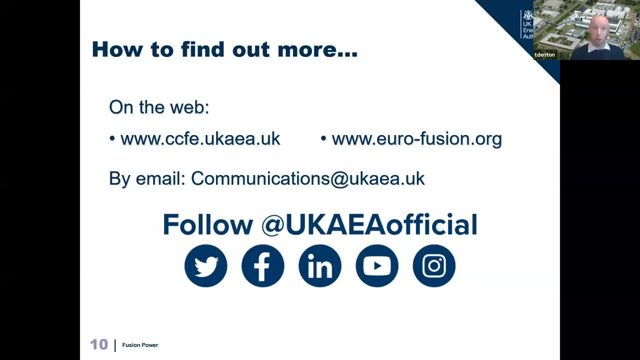 most interesting sort of things i've looked at so far in the last couple of years has been the real world of the job. so i think in the last couple of years i've been looking at capabilities mapping for model engineers and in my work not particularly the platform details of that i've 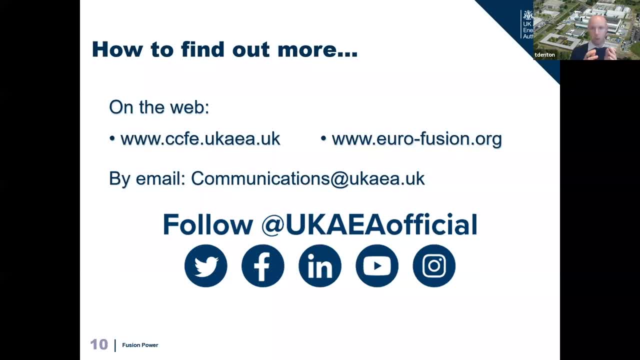 been looking at is the fastest moving technology in the world. i've been working with a huge number of companies in the world, and the number of companies that we've worked with since i joined this program 18 months ago was looking at capabilities, mapping through the life cycle of 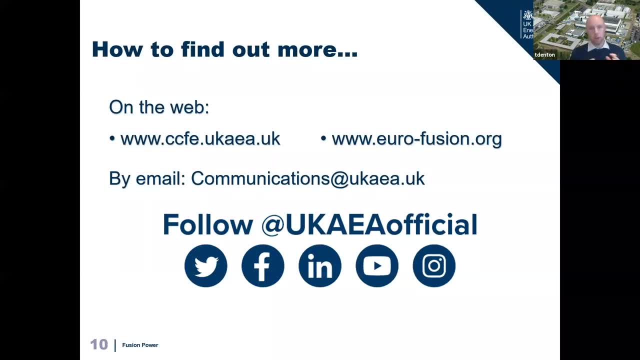 the program and how you move from heavy r? d to early stage design to detailed engineering, design to design finalization into program delivery, and each of those require different capabilities from the sector. um, if you're going to set up a new msc program in digital engineering, what course units? 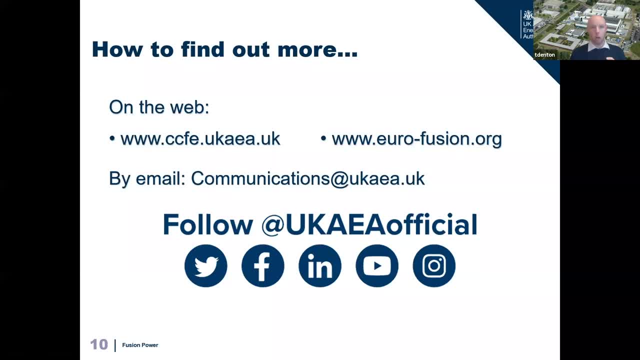 should it cover in order to ensure the graduates get their ground running the road? um, look, i don't know what i'm doing, but i'm just going to go and talk a bit about the program, a variety of different. Look, I don't want to get that wrong. I really don't want to get that one wrong, because that sounds to me like you're looking at something that could be extremely interesting. 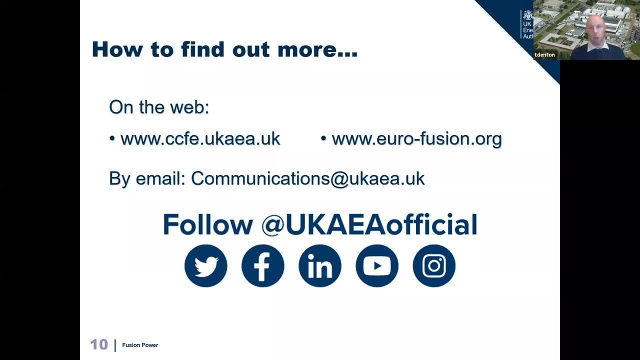 And digital people. you know we have the whole capabilities where digital fits- digital modelling, digital engineering. I'm sure they can give you really strong advice. So please do drop an email in to the address on screen that folks from comms team looking. please send that through to me and I'll work on that with our digital team. 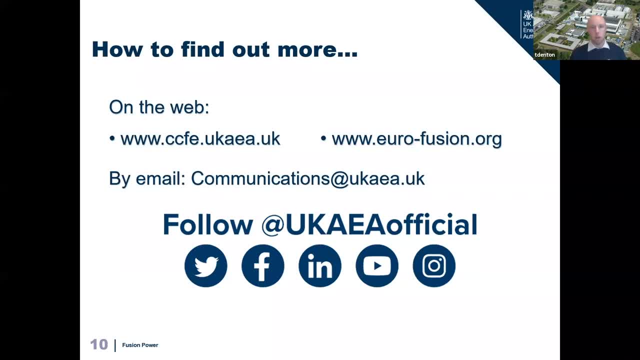 So has CERN a role in UK fusion nuclear? We've obviously got collaboration CERN. I don't overlap massively with CERN. Nick, if you're still on, I saw you pop up in comments earlier. I don't know if you can hit an answer to that in comments, because I'm sure you're far better equipped than I am to answer that question. 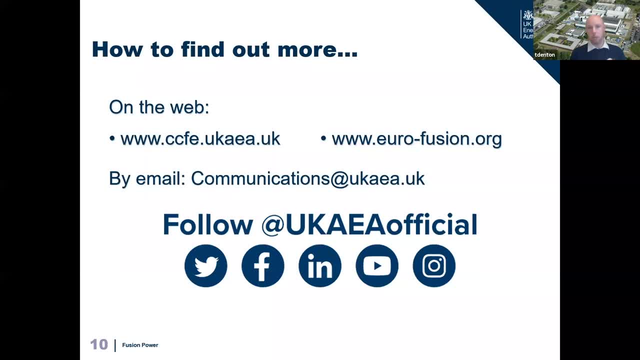 It's an exciting piece of infrastructure for sure. But, Nick, if you could pop an answer in the chat box, that'd be great. Thank you, Do we think fusion power will suffer any PR political issues from being established? Oh, that's a cracking question. I've spent a lot of my adult life working in fission power right, So I fundamentally do believe that fission's got a crucial role to play. 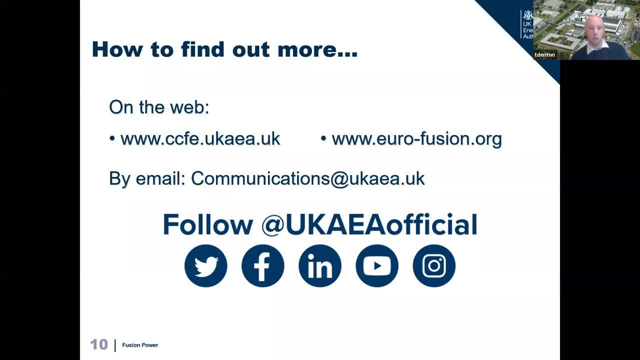 And when I worked in fission power, what you found was that I think polls for the Trade Association showed something like just over 70% of the British public were supportive of fission as part of a balanced energy mix alongside renewables, And that was probably two years out of date. 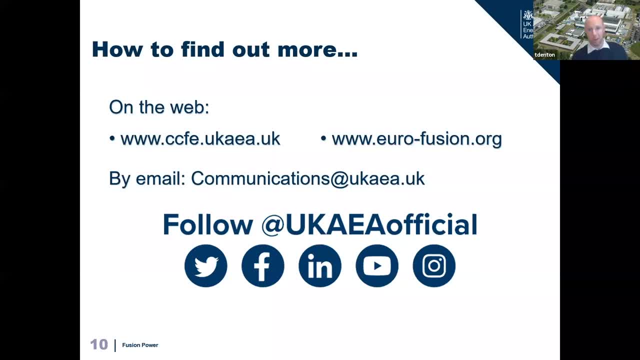 What you also find is that, round fission stations, round fission infrastructure, you have huge support where you're seeing familiarity, comfort with the technology and, of course, a significant socio-economic impact as well. What you see, then, is further away from those sites, and certain communities are concerned, obviously based on the waste and on the accident scenarios that can come with that. 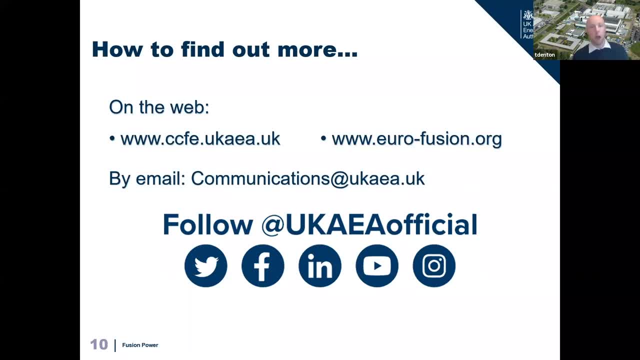 Now look. fusion is fundamentally different from fission. We do not have the same waste profile. We do not have the same spent fuels. We do not have the same fissile materials. We don't have the same length of life in our waste. We don't have anything like the same accident scenarios. I think one of the best things ever put to me was that the fission reaction, once it started, wants to grow and the job of the plant is to contain it. A fusion reaction, once it started, wants to stop and the job of the plant is to sustain it. 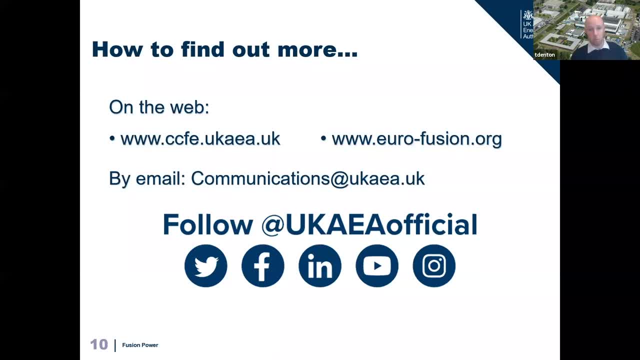 And I think just engaging on that point alone with the public will help. Look, I started life as a corporate communicator And I really do believe that when you're bringing forward either a piece of infrastructure or an industry, you need to have a frank, mature, clean dialogue with all of your audiences. 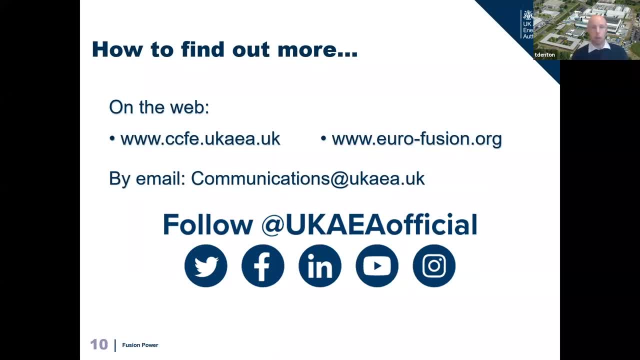 You need to be open about the challenges you bring and to be clear about how you resolve them. I want to put that in simple lay language: not to say you simplify the issue, but you speak honestly and clearly And I believe then- and my experience tells me- then your publics will usually come with you if your case is strong. 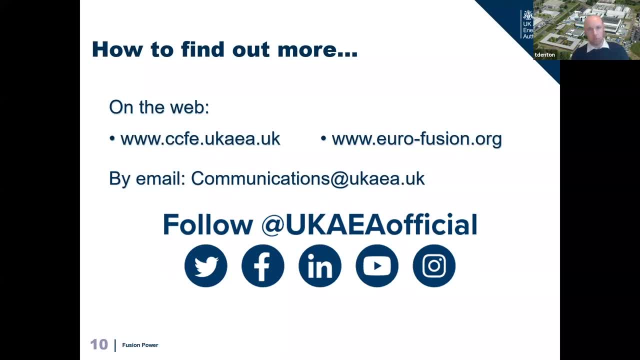 And when I look at fusion- potentially limitless, large-scale low-carbon energy, sustainably fuelled with low-level and very manageable legacies, low-accident scenarios- I think the case is extremely strong. I think the case is, in fact, incredibly attractive. 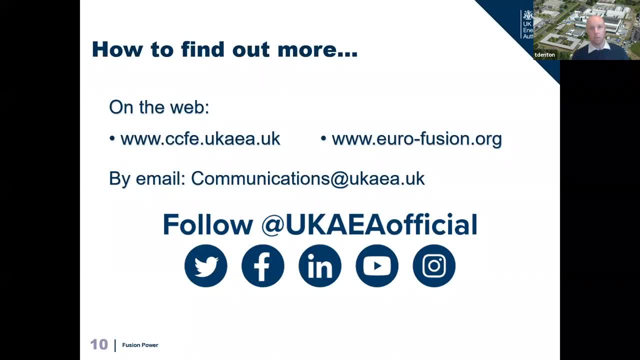 And therefore I believe if we have that open, honest discussion with the public, we've got a very good chance of securing sufficient support to deliver, And I think that's a very important part of the programme and indeed to be a very popular part of an energy mix. 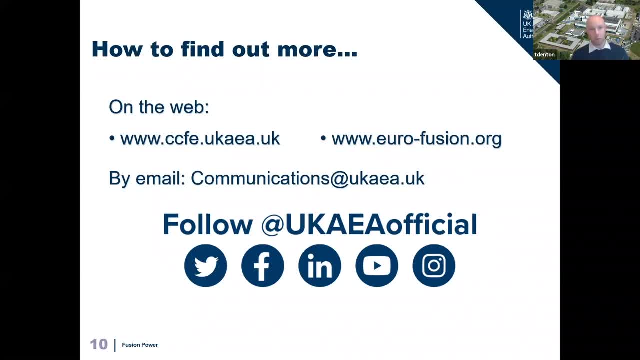 The challenge you raise about overlap with fission is of course a sort of tactical issue we'll need to address in those early years. I hope that answers that question. Given the focus on achieving net zero, is achieving a similar commercial viability with nuclear fusion compared to a conventional power station actually realistic? 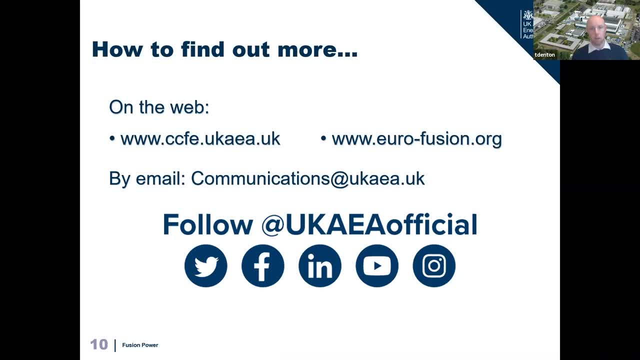 Should there be an acknowledgement that this will actually be less commercially viable over the achievement of net zero? So I think what's being asked there is: is fusion less commercially viable than other energy technology? I mean, look, of course, at the minute we're not in a position where we can bring products to market immediately. 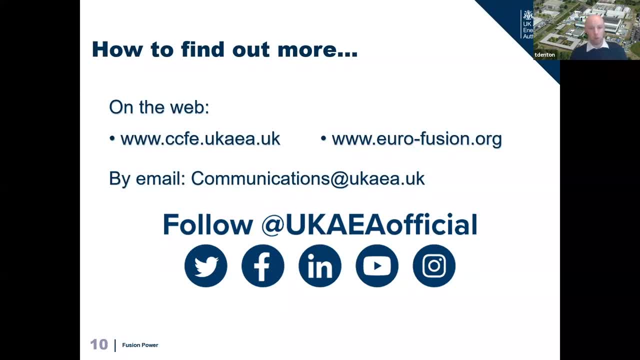 I think when you look at the nature of energy technologies on offer to the country, there's a number of options. There are very tried and established. tried and well established, fairly quick to deploy, but very carbon intensive generation methods. I think society, and particularly the policy environment, has decided that's not the long term future. 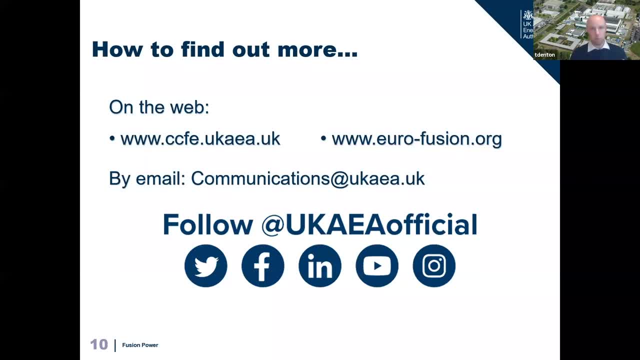 You've got renewables, which are a wonderful technology that have come on leaps and bounds, not just in their technical capability but in their price point- Phenomenal progress across the last 20 years- and they will be, and should be, a vital part of the UK energy mix going forward. 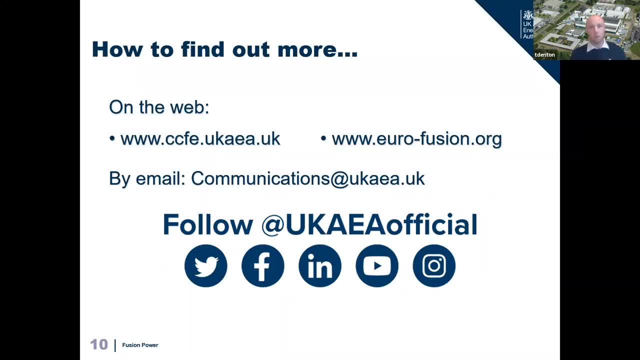 You've got nuclear fission which provides, Depending on the day, something like 20% of the UK's electricity and a vast majority of the UK's low carbon electricity has a role to play. I think where fusion sits alongside that is being an option for the future. 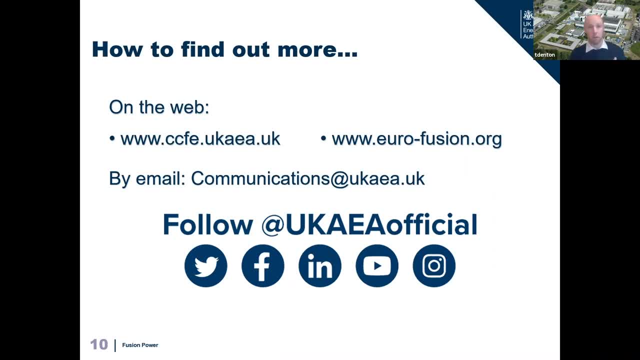 I've talked about expanding energy demands, potentially expanding electricity demands in the latter half of this century, And we believe the case is that fusion provides such a capable, credible option for that period that it's an absolute must that we investigate and research this now. 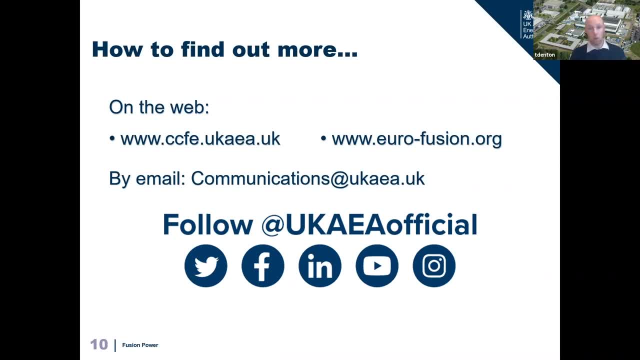 And the time, effort and resource spent on fusion are very well justified against that market context. Next one: I spoke at the point about the role of industry for STEP. how do we grow UK industry to maturity needed to deliver a power plant? Well, STEP did so. we do need more than just the Ministry of Health. Industry Supports Fusion. 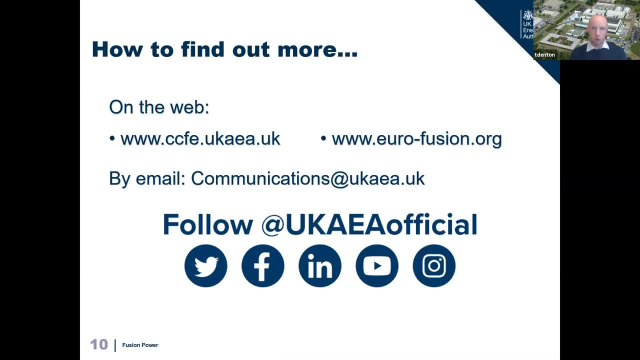 Okay, yeah, so you're right. We absolutely need the sector to grow alongside The top level programmes and let's be clear, that is not just for STEP to do. STEP is one sort of stimulus and one client base. When I talked about the role of STEP and how it sits alongside other programmes, I talked about the need for a breadth of clients. 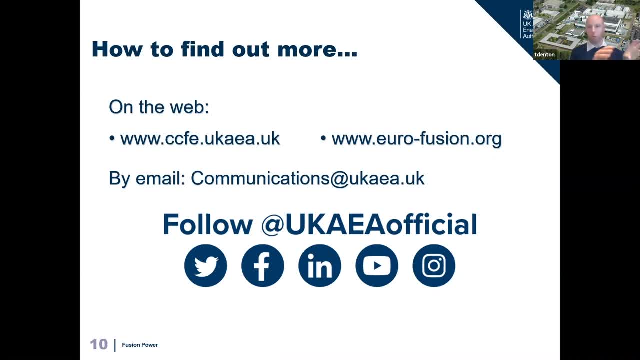 And if you look at any industry, fission is an easy comparator: The more projects you've got going on at the top level, the more there's a business case for the supply chain to invest in people and equipment and training and development to be a supplier in that field. 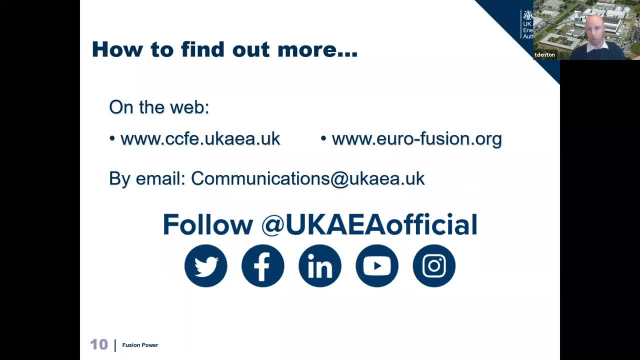 So I think, as you see fusion coming forward- And let's be clear, There's some fantastic private sector projects going on as well, alongside other very exciting UK AEA projects and, of course, ITER. I think there is an increasing basis of clients there who will want to work with the sector. 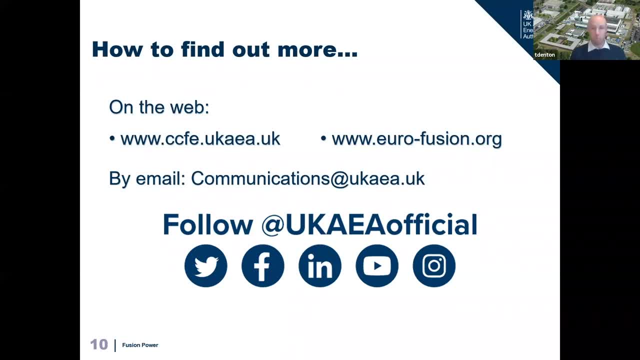 That's a strong stimulus. But look, if you go back to the very core mission of UK AEA, not of STEP but of the authority, growth of fusion in the UK, with the scientific benefits but also the economic benefits, It's key to that. 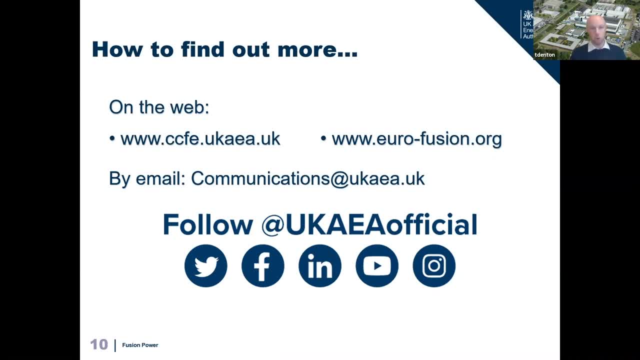 And I think we as an authority need to keep focusing on providing opportunities, understanding and engagement opportunities for the supply chain at every level to get involved here. And the reason I talk about every level, by the way, is there's some, you know, there's some really exciting and interesting niche SMEs in fusion who do vital work. 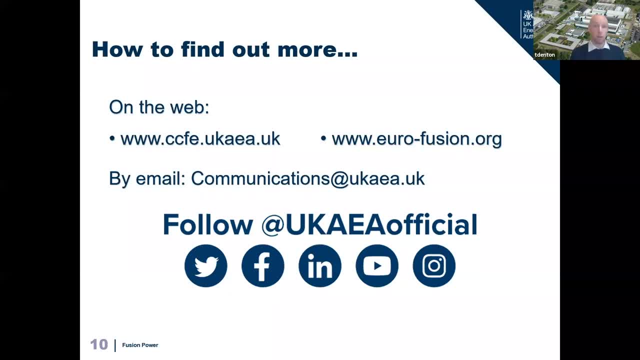 But also when you pull back and look at the plant, a lot of it isn't necessarily fusion specific. the barriers to entry for existing companies may not be as significant. But also when you pull back and look at the plant, a lot of it isn't necessarily fusion specific. the barriers to entry for existing companies may not be as significant. 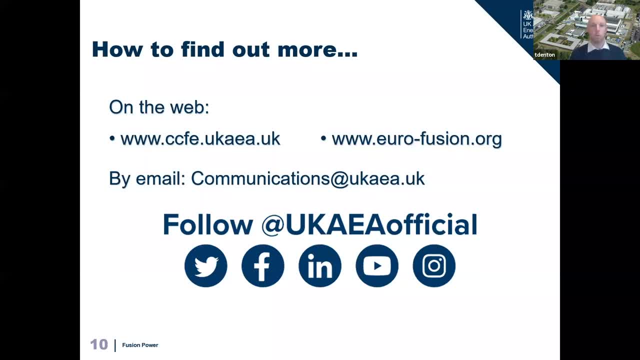 But also when you pull back and look at the plant, a lot of it isn't necessarily fusion specific. the barriers to entry for existing companies may not be as significant As those companies might perhaps believe when they take a look at the sector from afar. 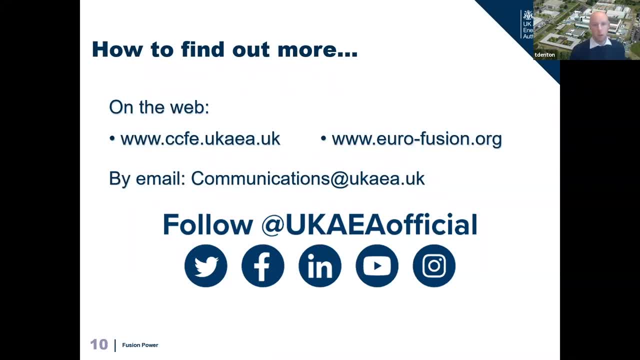 What are the current projections on cost per megawatt? Will fusion be able to secure funding? If so, will it drop? So we've not done cost megawatt predictions as of yet. It would just be at this stage of design maturity. it would be premature for us to try and forecast that. 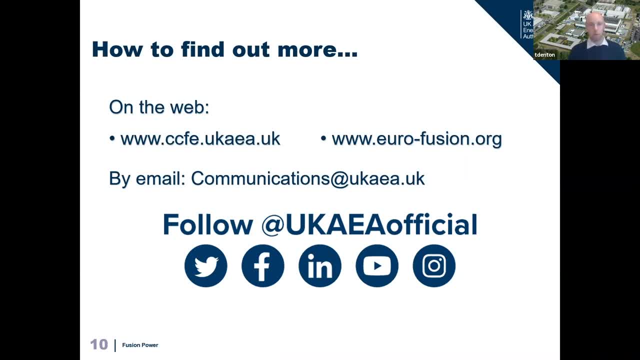 What we're focusing on is designing with a cost conscience, Bringing those costs down To the right level and then for that would enable us to have the right cost- cost per megawatt when it comes to it- And do I think we're competitive if, if- renewable costs continue to drop. 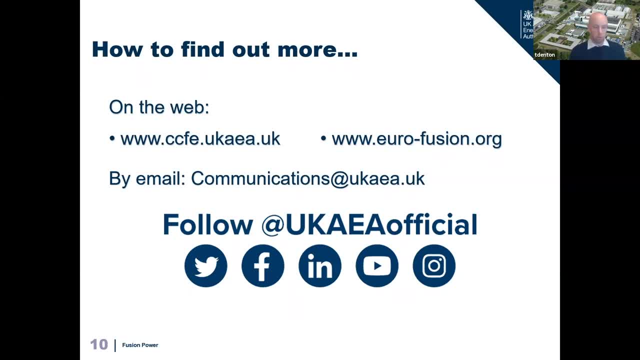 Yeah, you know, I think research after research shows that actually what, what the country and the world needs is balanced energy mix, A range of generation sources coupled with the right approach to downstream mechanisms. We do need to be on a par with other technologies, but I don't think the energy market. 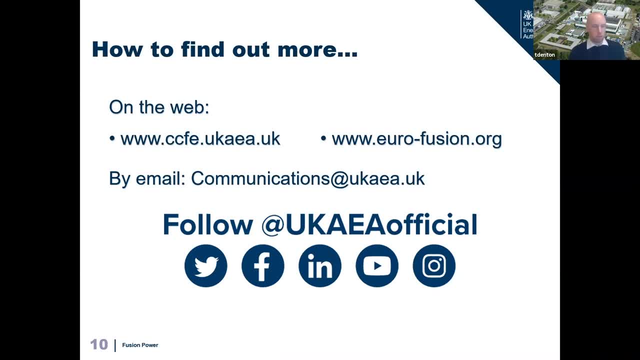 Has ever been as simple as saying: it's a race to the bottom to be cheapest and you know that then you dominate the sector. I think it's about being at the right price. right price, competitive and part of the overall mix in terms of policy needs, societal needs and more. 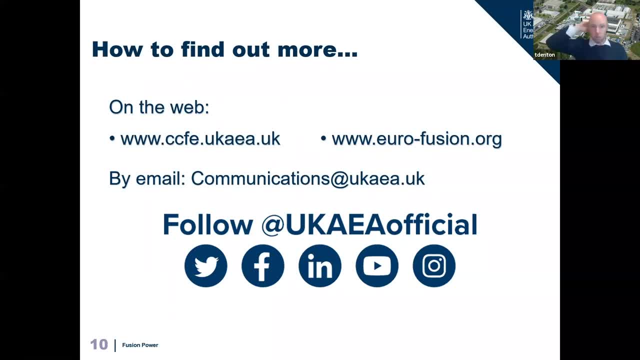 Current design status of STEP. there are many challenges facing us as a tea based power plant, plasma exhausting, tritium breeding. how can they be tackled? Will there be experiments planned for tackling the challenges? Yes, there will. Tackling those challenges is what we are all about. 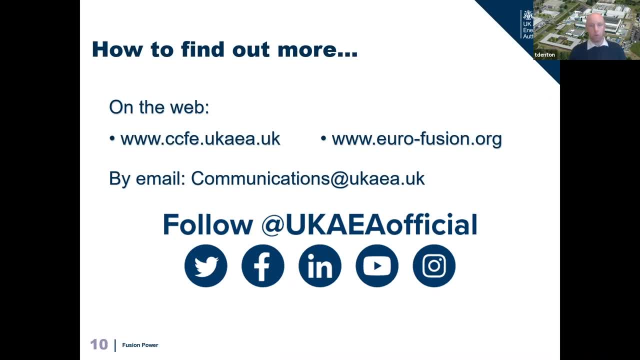 Obviously, plasma heat, Exhausting and things that master you offers a lot of learnings which are really important. tritium breeding is, of course, something that the sector as a whole has looked at many times, and we've got research programs underway. 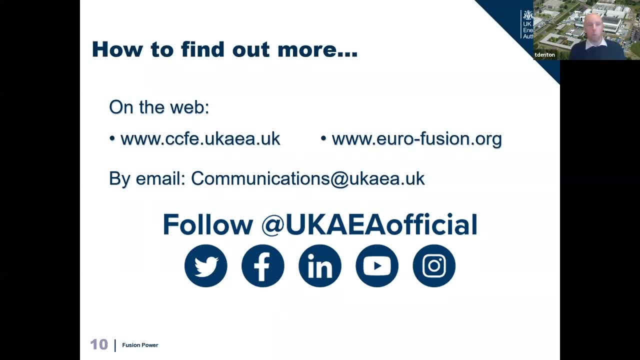 The experiments. we do. that and the fact that those experiments are hardwired into design programs is really the essence of step. It's overcoming these design challenges in a way that is design led but research informed, And we think that offers us the best route to to our outcomes. 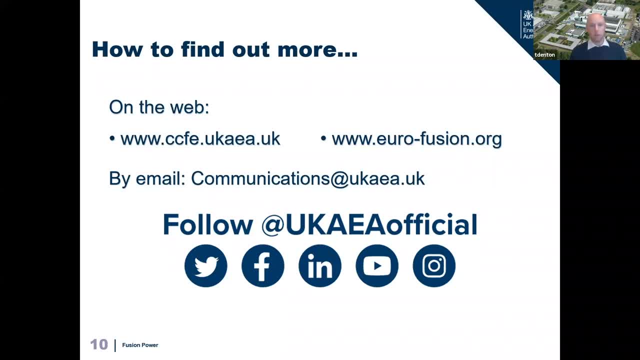 What's the environmental sustainable target for the project would like to achieve? that this is. this is inherently a sustainable program in our eyes. Now we know that what we're talking about is bringing forward large scale low carbon energy. We know that sustainability and design is right. 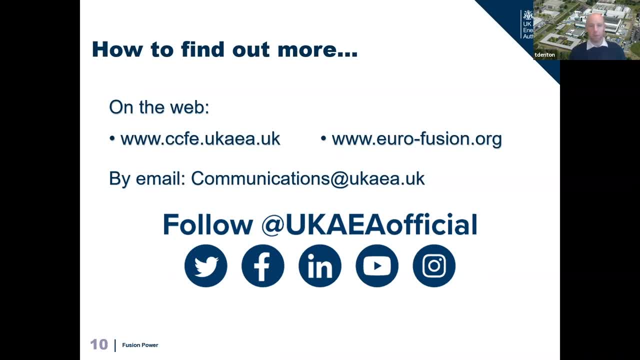 If you cramming design with loads of extraneous metal and concrete, your sustainability credentials fall And of course we'll look at that as well when it comes to designing and developing the site. We haven't got a benchmark target quite in the way you frame it there. 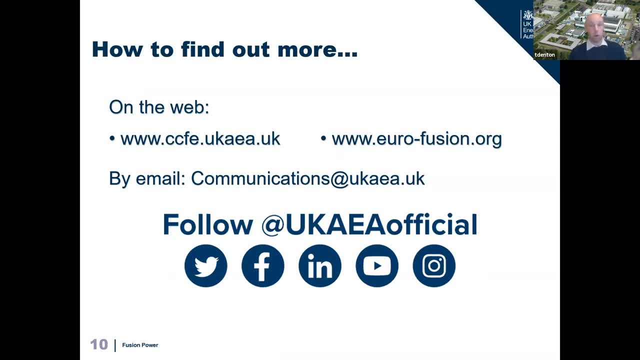 But there are a number of environmental criteria, both regulatory and non-regulatory, which will will drive work as we go forward. It appears to be a lack of available instrumentation at work in fusion environments with a neutron impact And, if ever, been made with interested parties to develop the applications. 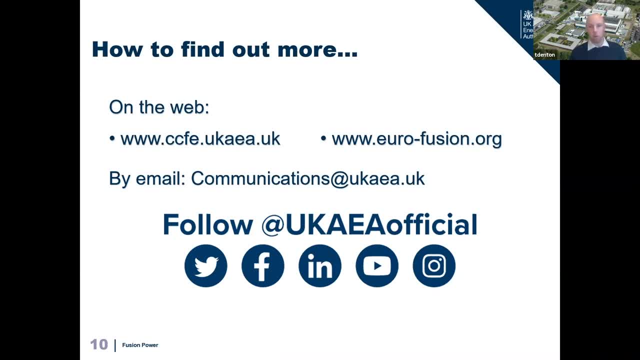 Really interesting question. I would imagine that our investor component team would be looking at exactly these points And, as I've said a number of times, materials research is vital To that, both to making sure you've got things that go in, but also things that can have the longest lifespan once in. 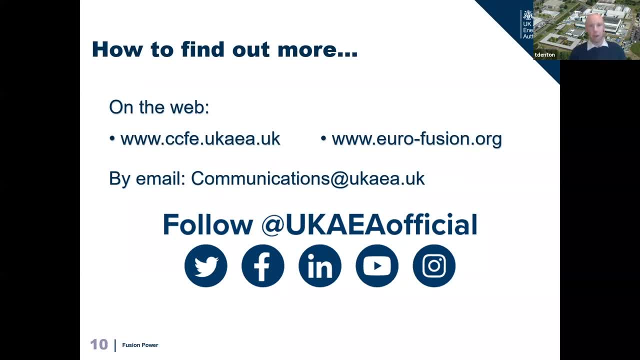 At this point of design maturity I would imagine we're probably still tackling some of the bigger ticket items, But of course that's going to be a really significant package of work as we go forward. If you want more on that, I'd be delighted to link you up with our investor components lead, who is rather fantastic on these things. 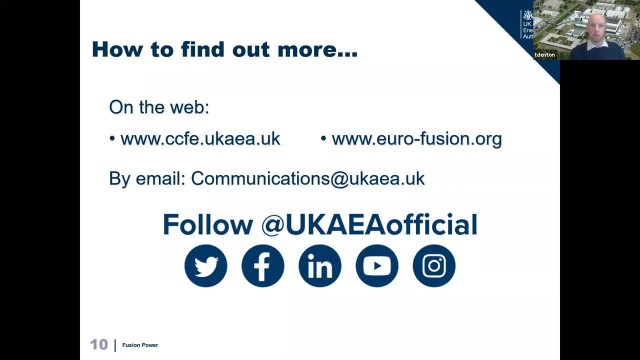 So you know, do drop us a note through through the contact details Shared. Do you have any thoughts on how future fusion power plants can be made viable for countries who don't have the university's institutions that develop the technical skills? That is a really interesting question. I think we all know that- to be commercially viable. 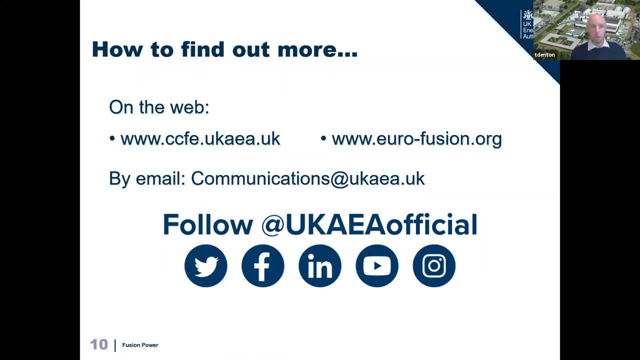 but also to have the maximum environmental impact. we want to see fusion deployed as widely as possible. Right, And as widely as possible is not just here in the UK. Fusion is obviously very different to fission in terms of its requirements. So safeguard and safeguarding regimes, regulatory constraints, but they are not non-existent. 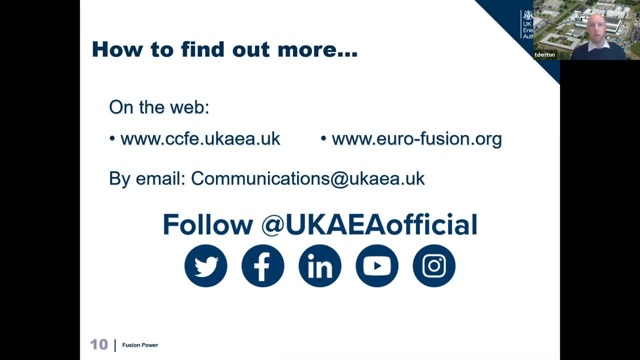 So I think our priority is to design a plant that works, to design a plant that's capable, but also, of course, to design a plant with the biggest breadth of market applicability it can have, And that would mean a plant that, as far as possible, can be exported and deployed in areas not necessarily familiar. 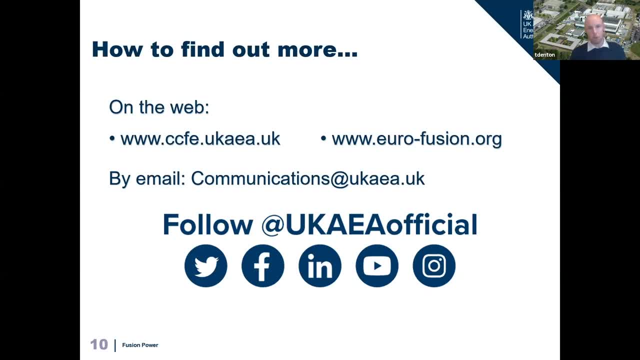 And of course, that would not just give a power station. It would also provide opportunities and a stimulus for investment in skills and capabilities and growth In those regions, which is an added benefit. But yeah, we're really clear that you don't get the scale of environmental impact. 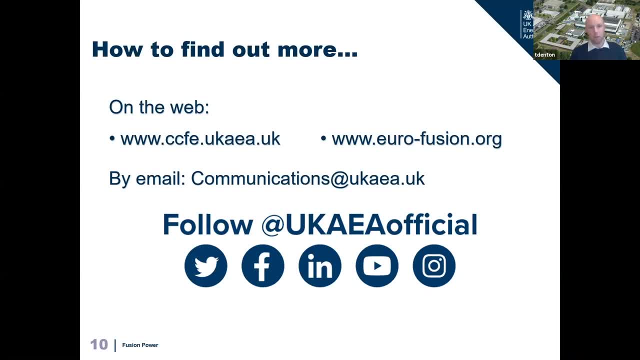 we want, if you only deploy in areas with massive fusion academic knowledge. Does STEP have to be built on a nuclear licence site and will it be built in the north? Fascinating? No, So nuclear site licences don't transfer with ownership, So it would not have to go on a current nuclear licence site. 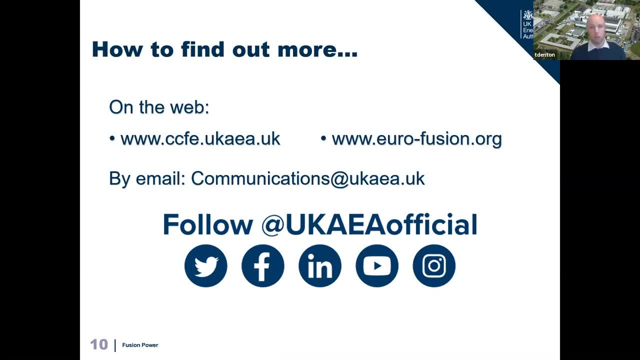 Will it require a nuclear site licence remains to be seen. The regulatory framework will have to be designed, Decided by government. Obviously, Cullum operates under a system that is HSE, an environment agency, therefore not nuclear site licenced. 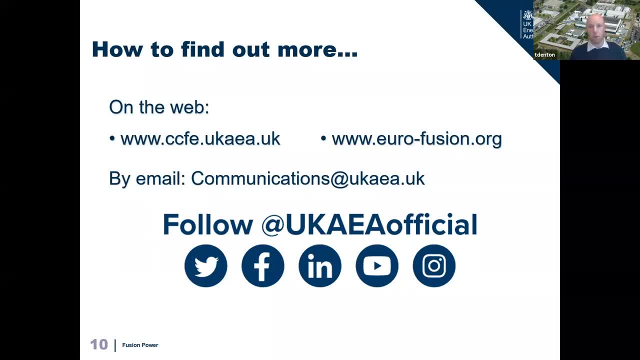 Will it be built in the north? I don't know. We'll run a really fair and transparent process, As I've mentioned publishing details later this year through which we will seek candidate sites and ultimately a recommendation will be made And that will be a subject for Secretary of State to make the final choice. 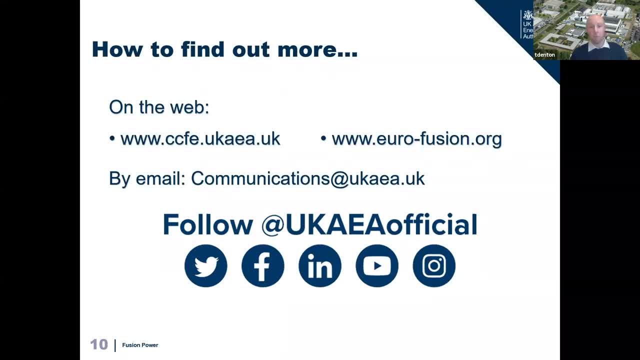 Any thoughts on international collaborations concerning STEP? Yeah, lots. You know there is a need for collaborations with academia, supply chain third parties and obviously they're already global. If you're looking at state to state international collaborations, I'm not quite sure whether that's where you're going with that. 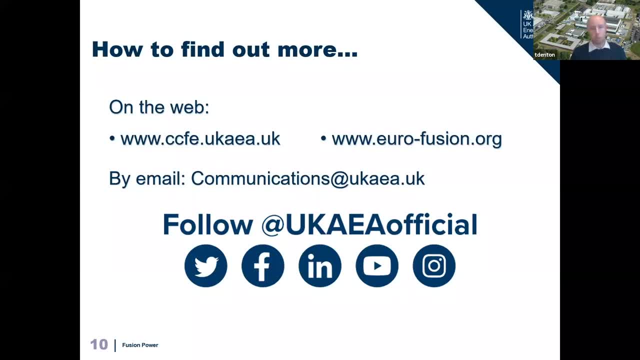 It's not part of the current plan, but obviously fusion's got a long and rich history of collaboration. But let's be clear. It comes back to what I said, I think, in my second slide. There is no one entity that can deliver this on their own. 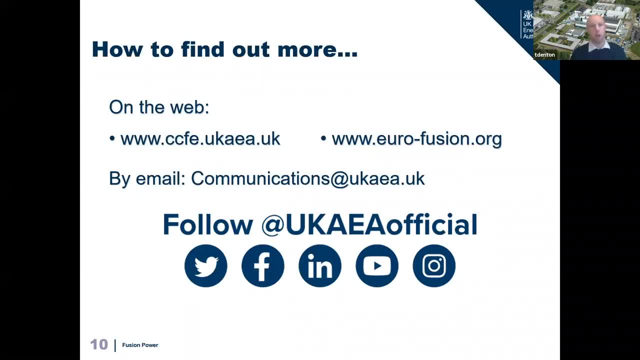 There's no one entity that can crack this nut. We will need collaboration from academia, supply chain and beyond And absolutely are already working to get that. Apologies for slightly cantering through these. I'm aware I've got 22 questions and only nine minutes. 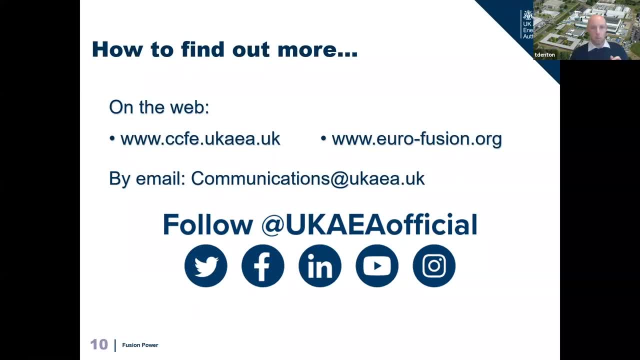 So I'm doing the best I can. Are we looking to develop a process to keep the cost of fusion minimised to ensure it's commercially viable? Yeah, absolutely, We want this to be commercially viable. The key to that is in this design process. 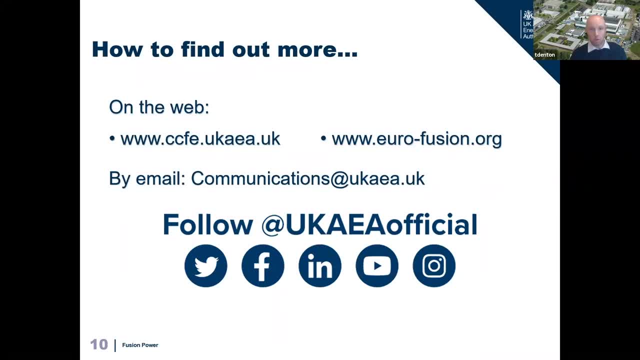 We need to make sure we bring forward A a piece of kit that works, Because if your power plant doesn't produce power on a reliable, predictable, stable, informed, reliable basis, you just can't be cost competitive. What you then need to do at the next level is try and keep the capital cost of that down and the lifecycle balance of rate of return up. 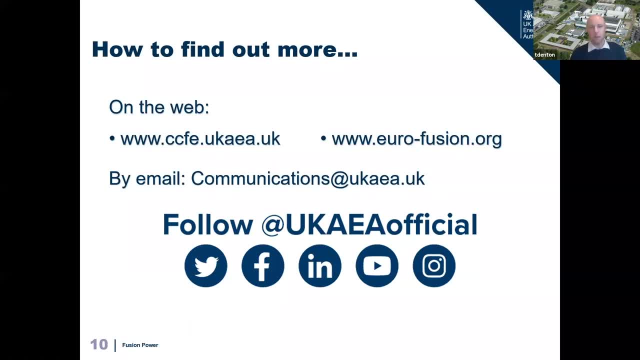 This is fairly straightforward in things. It's fairly straightforward in theory and, of course, extremely challenging in process, And it will come down to design constraints and some tough design decisions to be made across the next five and then ten years. How do you think the lack of a fusion-specific regulatory body will impact design? 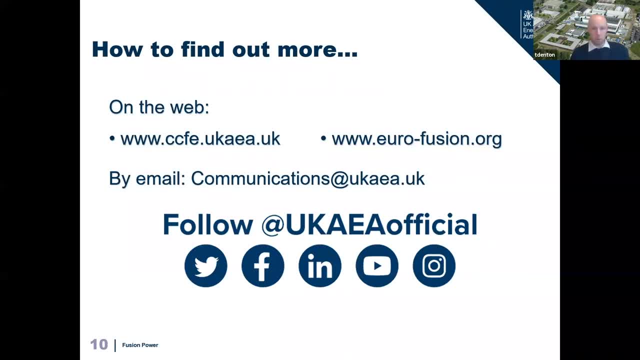 Are there concerns that over-regulation could slow the pace of deployment? Excuse me, I'm getting what's called Zoom voice, where you talk on conference calls all day and lose your voice. Look, we need a clear, stable regulatory regime. 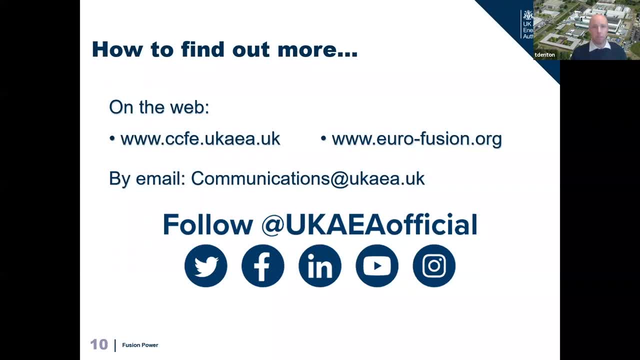 That's obvious. Government understands that And, of course, we are currently regulated at Column by the HSE and the Environment Agency. Obviously, regulation needs to be proportionate to the scale of risk. Regulation itself is a good thing because it provides a clear operating environment. 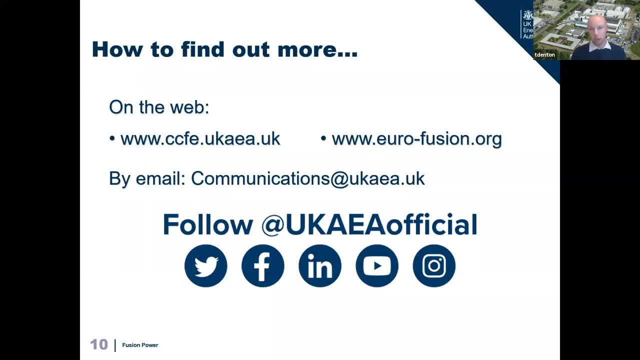 And also it gives third parties confidence in the maturity of the technology in the sector and it gives you public confidence. It's about making sure, as I say, that that is the proportionate regulation in the right way. I hope that answers that. 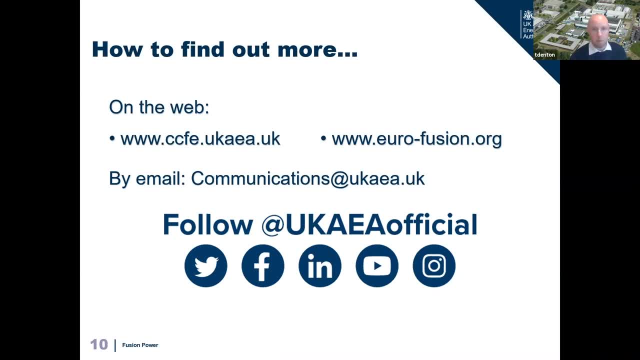 Expected output in megawatt E TBC. we have yet to confirm the detailed output in megawatt electric. We don't expect this to be a full commercial scale plant from the off. We do expect it to be consented under development consent order type arrangements. 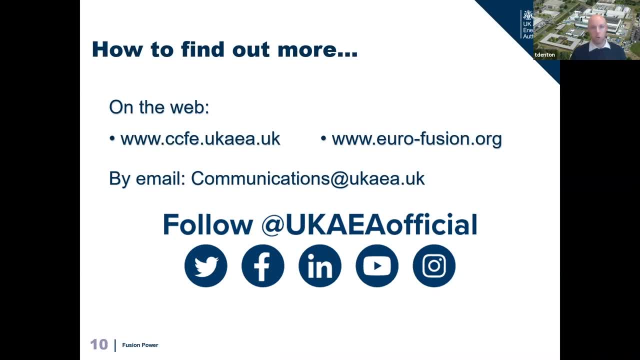 And we'll work on that And I'm sure we'll have more to say as we proceed through Tranche 1.. To add to the questions: will the step design process take advantage of technologies from other industries, including fission, to minimise the costs? 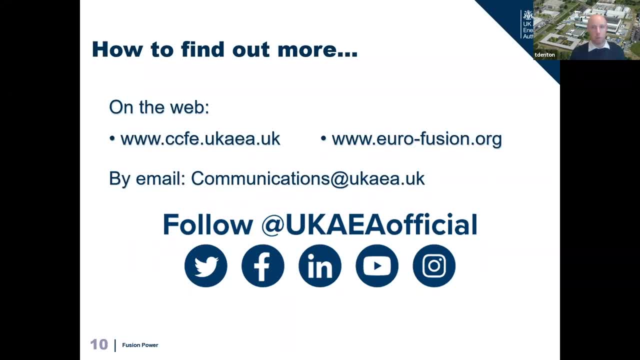 If so, is there a process being developed to ensure this is learning for other industries? I mean, yeah, absolutely. Nobody wants to reinvent the wheel right. There is no glamour and glory in ignoring things that have been done and are public sourced and well known already. 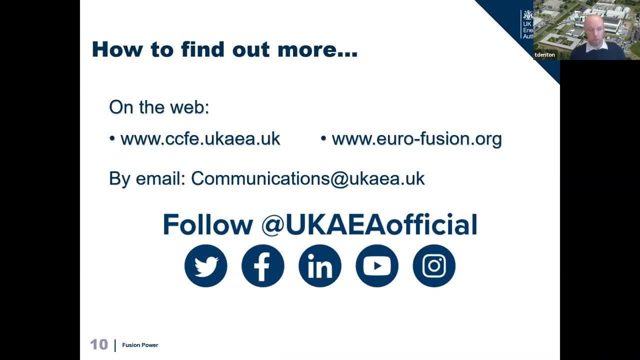 I mean. a lot of that happens naturally by osmosis, in that you appoint good people to these leads and they understand their sector And they understand the innovations in those sectors. There's also a wealth of public domain information published by public and private bodies about this. 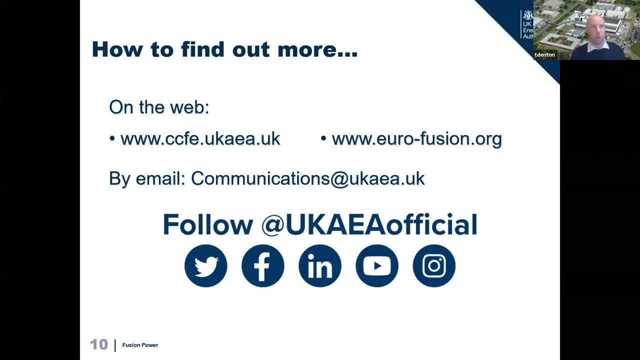 In terms of process to capture learning from other industries? it's a really interesting question. I don't think we have. There's various UK AEA-wide activities to capture innovations And we've done a couple of smaller supply chain innovation challenges. But you're right. 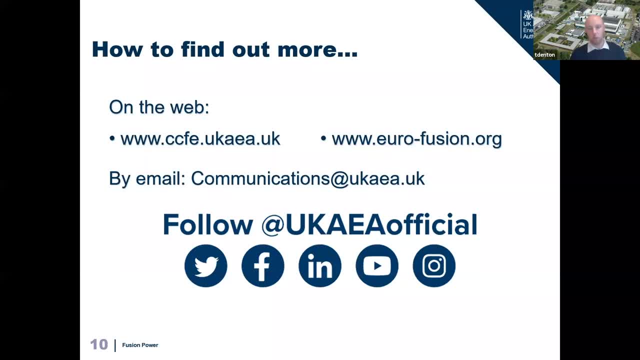 There's something interesting there about making sure we have a sort of bespoke portal to make sure we're learning from the best of industry already. So I might take your question and turn it into advice, if you'll forgive me for doing so. Not a question as such, but a more comment about the less quantifiable benefits of big new technologies. 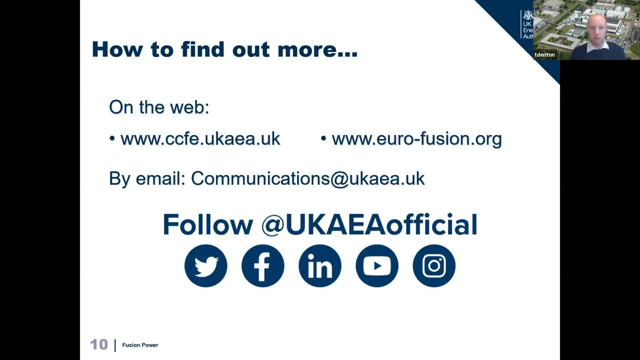 Won't go as far as quoting JFK. Oh, go on, go as far as quoting JFK, But it is a similar challenge that's worth doing for other reasons. Newtons has much higher employment benefit compared to renewables. Yeah, I mean look. 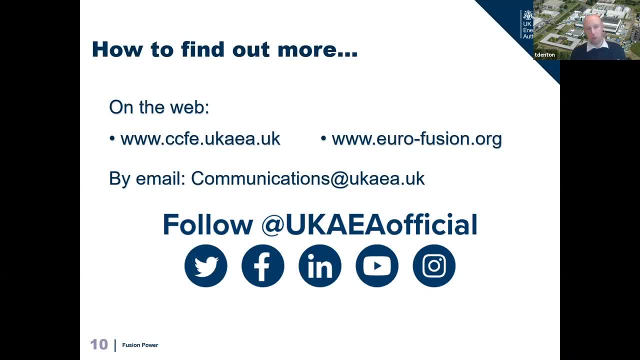 So, yeah, there's a whole range of benefits. One of the key factors of this is spillover technologies. We understand that the piece of work we do might be applied to STEP. It might be applied wider in UK AEA. We might find innovations which aid the wider sector or further out into completely unrelated non-energy sectors. 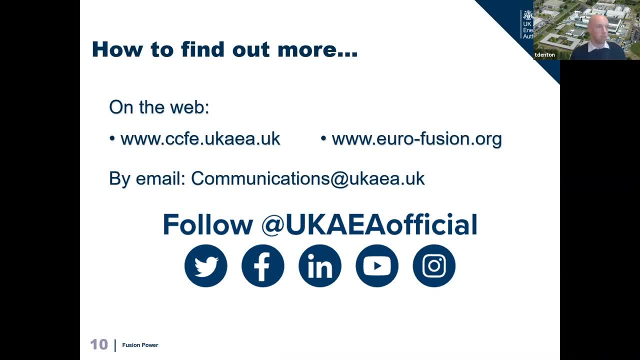 Investment in R&D has been showing time and again- including looking at UK AEA spend- to be a very positive thing. that generally adds gross value add- Gross value add to the country. We then, of course, need to capture that for our own aims. Nuclear has an employment benefit. Yeah, I mean. personally, I never get into technology versus technology. I don't see a win there. Ultimately, the country will need a complete balance of energy technologies. that would include fusion, fission renewables. 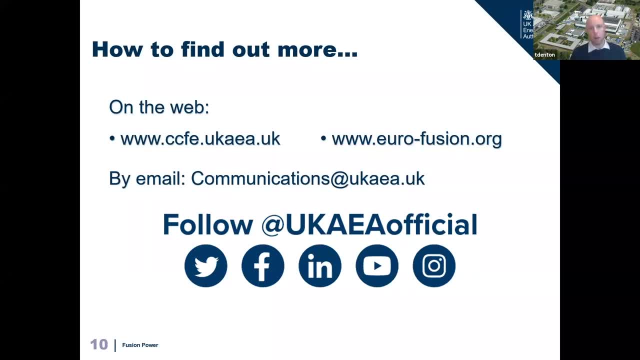 For the time being, it includes clearly significant component of fossil fuels as well. What we need in this country is strong capable supplies of low carbon energy And strong capable industries that deliver them and provide UK jobs in the process. Is STEP to be a demonstration tool or a research tool? 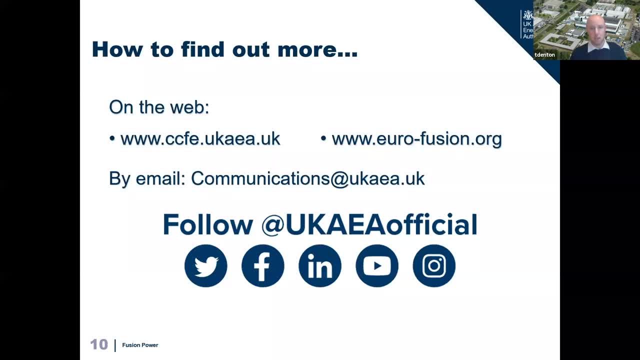 Look, STEP is a prototype, so it should demonstrate the capability and credibility of the design. It would, of course, also produce a whole package of learning and experiment opportunities and wider knowledge. So I think I'd say it's not a demo or research. 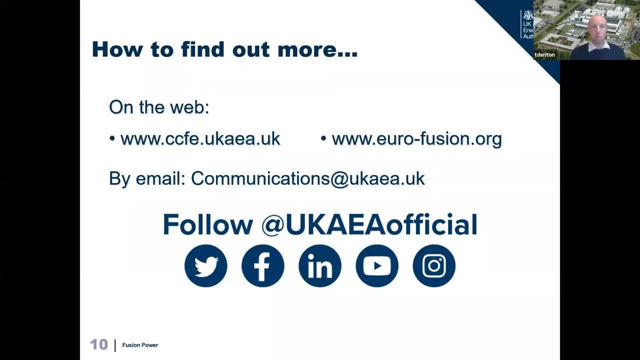 It's a prototype in that sense. How big or small is STEP going to be compared to ITER? Look, smaller is the starting position. Compact, spherical tokamak will evolve both our design and site layout over the coming years. And again, to note that anything we do will be subject to full planning consent applications. 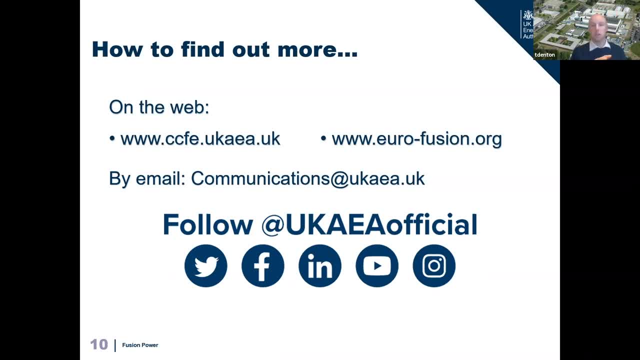 Right, I've got about two minutes to go. Just to say now that if I don't get to your question I'm really sorry. I promise I'm cantering as fast as I really can. Please do pop them in In email. 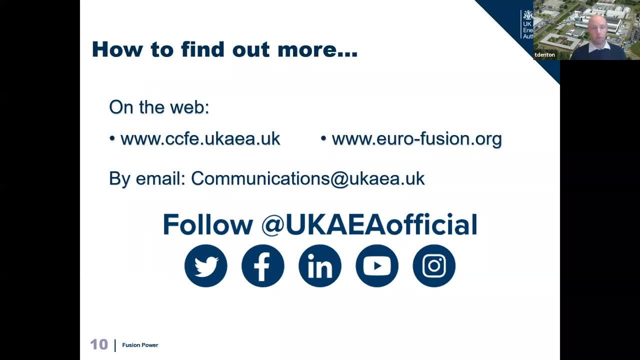 And we'll get back to you through our corporate comms team, But for the last couple of minutes I'll keep diving on. How detailed are the current designs? Are there any problems with machines? I promise what I've said. it's state to state operation targeted. 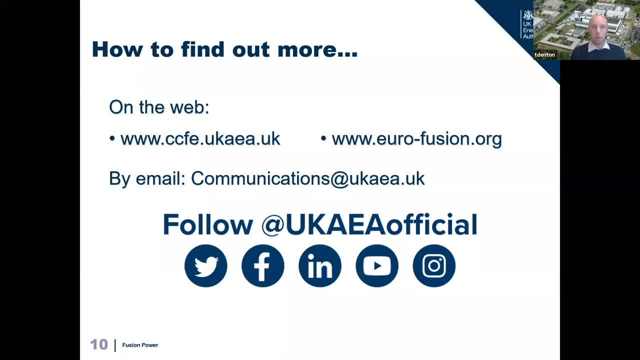 We're at the early stage. We've been working for about 18 months of a 21 year programme, So clearly the design is at a fairly early stage of maturity. Some aspects of the design are increasingly looking like they might be clear, But it would be wrong for me to pre-empt those. 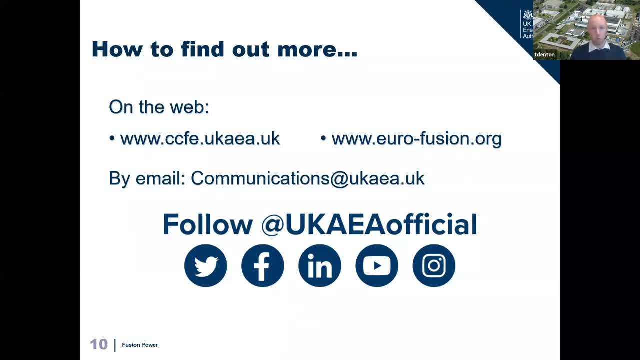 Obviously, there's some aspects of that We'll keep in-house whilst we're developing it. And yeah, there's clearly a number of ways you can operate this plant, either through steady state or pulsing, And they both have interesting attractions. 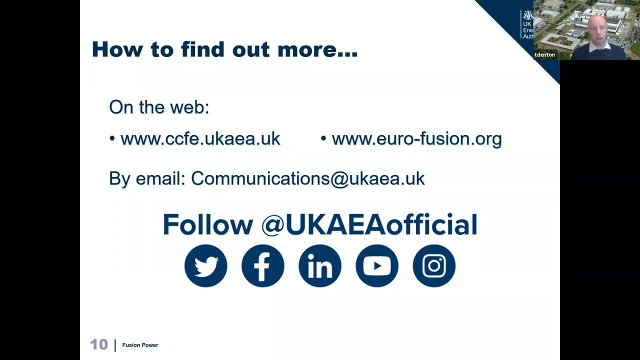 Will the CE marking process be involved in STEP project? Without a doubt, we'll need component accreditation and supply qualification. I don't know exactly what process that would be. Codes and standards are going to be a really important part of this, But yeah, when you're building any high value energy technology, 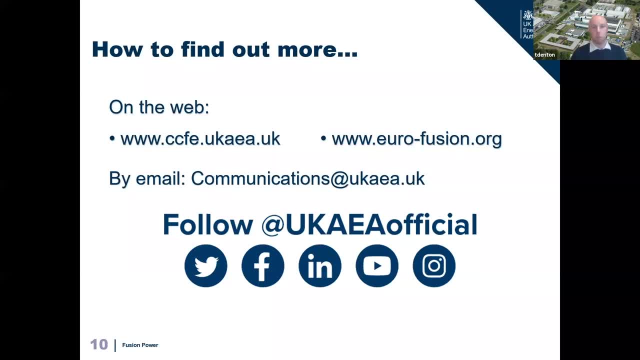 you have to make sure you guard against counterfeit and substandard materials, And code standards and markings are one way of doing that. Is UKA still interested in DEMO? Of course, fantastically so. ETA and DEMO are really important programmes. 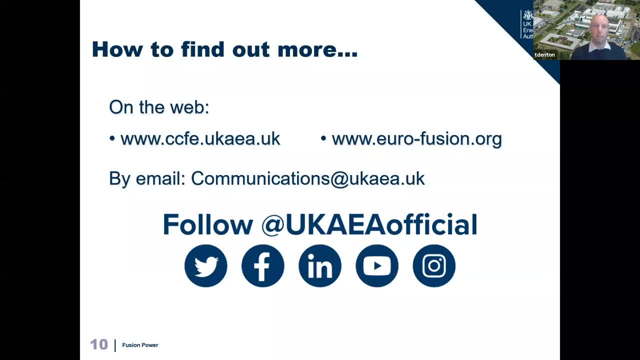 We've still got people very much working on them. We want to collaborate. They're really great, great pieces of work. STEP is, we believe, a helpful addition to the international collaborative suite of programmes. In no way is it, No way is it a replacement. 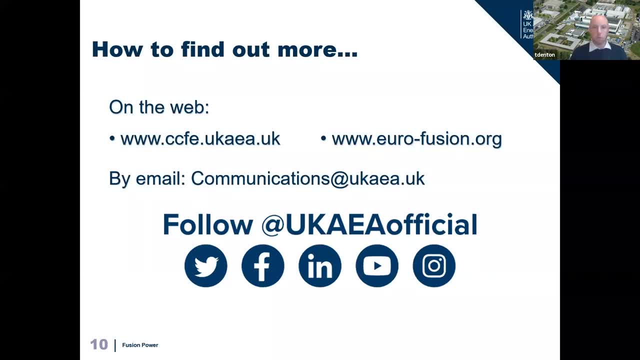 And I think that probably answers the comment below on ETA as well. Has the option of smaller modular STEP stations been explored? Was it meant to roll out? be useful for more locations? Yeah, it's an interesting question. Look, we want to bring forward a design that has the strongest market options in it that it can. 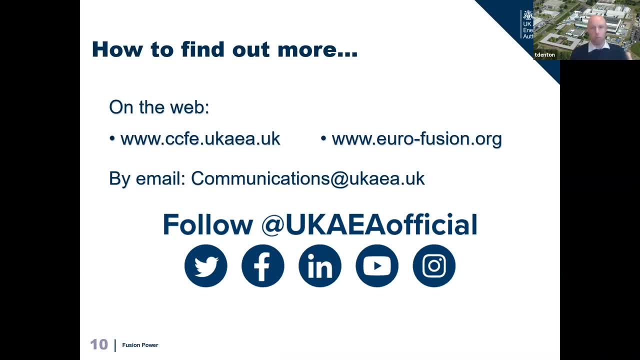 Look, I think it would be naive at this point, 18 months into a 21 year programme, to start saying we could do this derivative, that derivative. What we need to do is come to a really strong concept design. But of course we've got people looking at what energy market is driving towards. 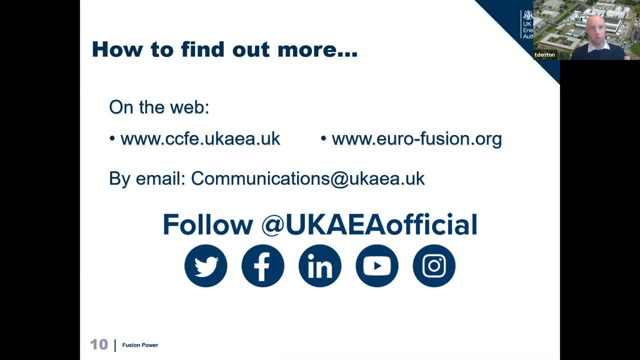 And you know, you could see clearly in fission space that smaller modular plant is currently viewed as in some ways more attractive. We want STEP to be as deployable as possible. It's the most honest thing I can say at this stage of maturity. 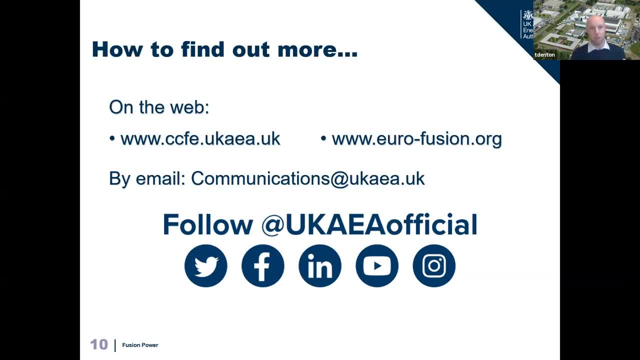 Ask me the question again in 10 years and I'd love to hopefully be able to tell you where we are on the court. Design and derivative designs also. Can you please recap the alternatives to STEP other than power generation? Look, there's a whole range of ways STEP could be deployed. 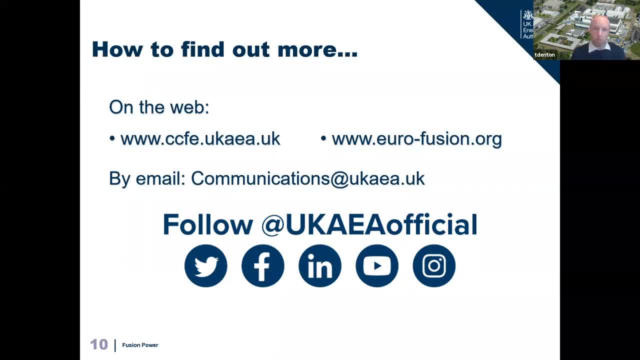 So the STEP plant will be the demonstrator, the prototype that will prove the principles of the design. But obviously there's a number of other uses. So power generation is one, be that for electricity, for hydrogen, And then you've got non-power uses like medical isotopes and things. 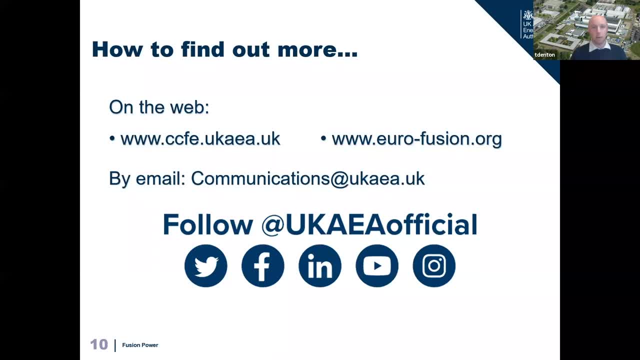 which are worth exploring and are very interesting as well. The priority now is to understand the design, understand what we can bring forward and research the market applications which might be possible. Look folks, I'm. you know I hate leaving 10 questions unanswered, but it is 2.30.. 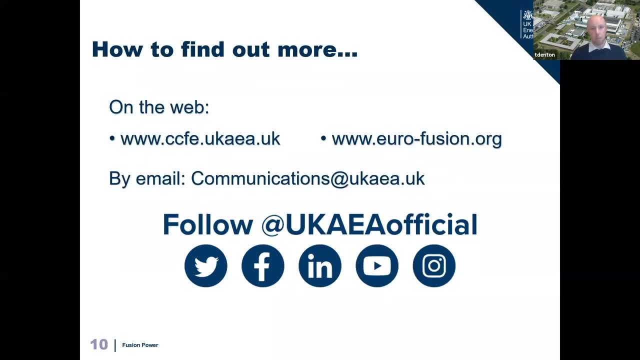 We are at the end of our time slot there. Please, please do pop them in Communications at AEAUK. You can follow us on all the social channels as well and find us on our website. Just thanks for taking the time.